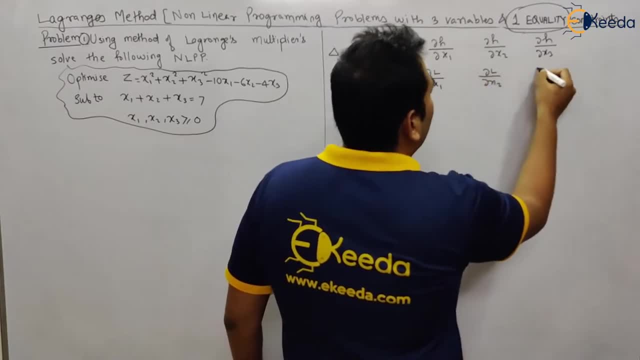 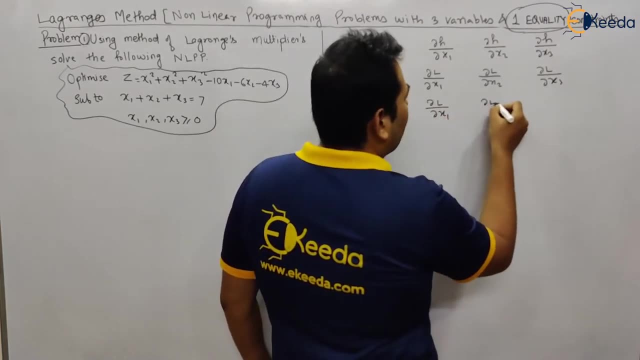 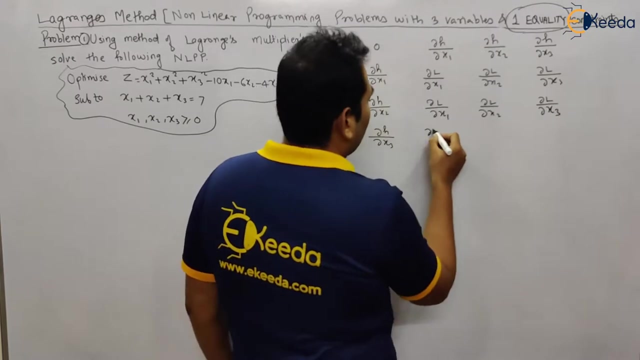 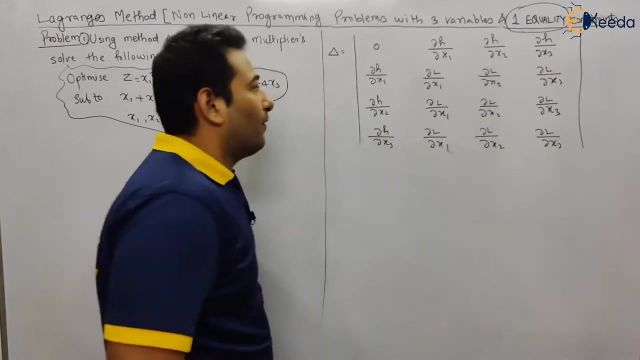 We are going to differentiate with respect to x1, with respect to x2 and with respect to x3.. Same thing I am going to repeat here. Same procedure As we made delta in the last problem. similar procedure to find delta here. What next? First, this row. we are going to differentiate. 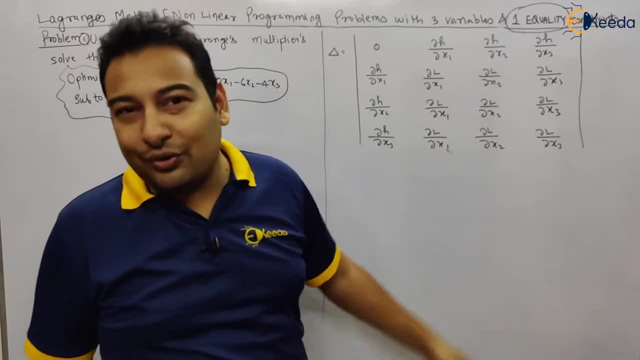 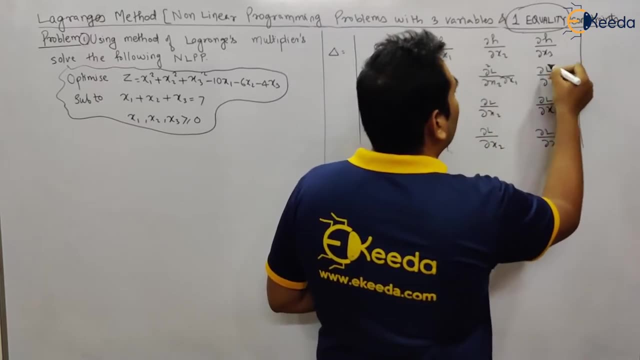 with respect to x1.. We are going to differentiate with respect to x2.. We are going to differentiate with respect to x3.. So this will be x1 square, This will be x1 and this will be x1.. Next, we are going to differentiate this row with respect to x2.. 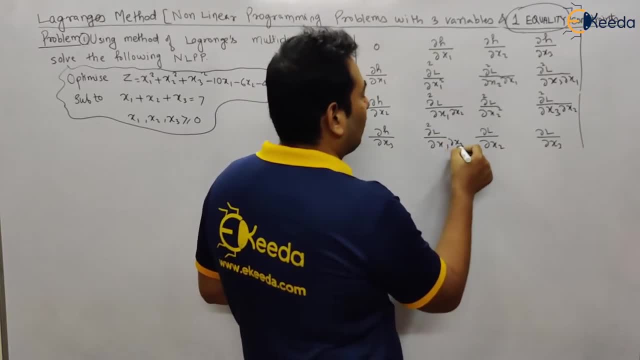 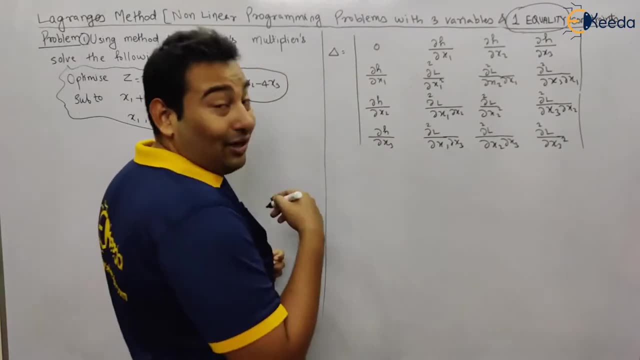 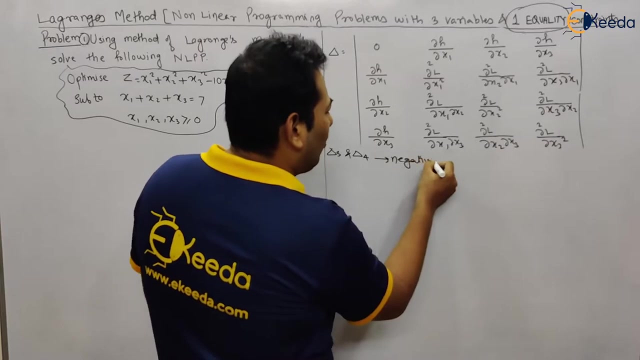 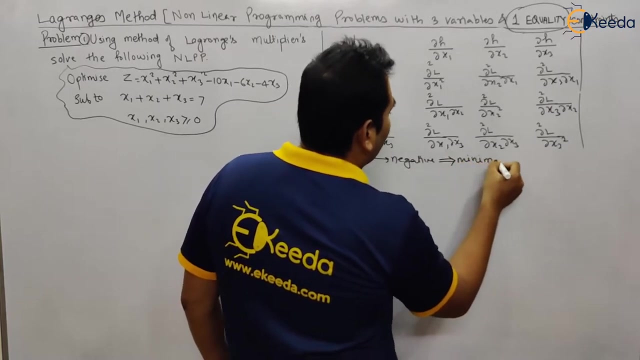 Next, with respect to x3.. this matrix is ready. now here there are two possibilities: delta 3 and delta 4. both are negative. we'll tell you what is delta 3 and delta 4? that we'll discuss later. if both are negative, then it is minima, and if delta 3 is positive and delta 4 is negative, 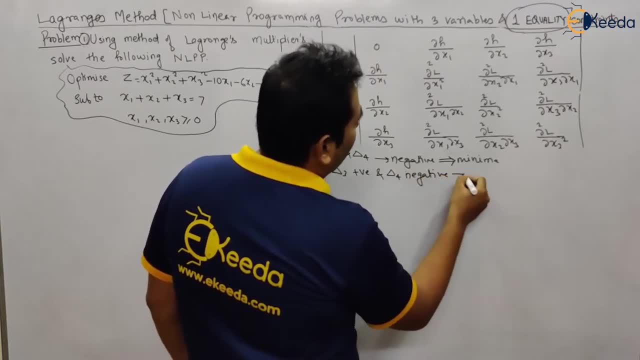 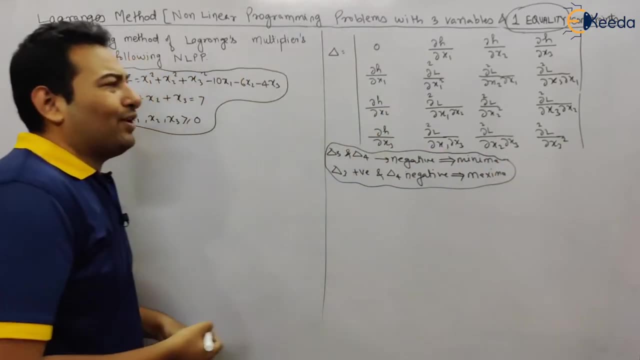 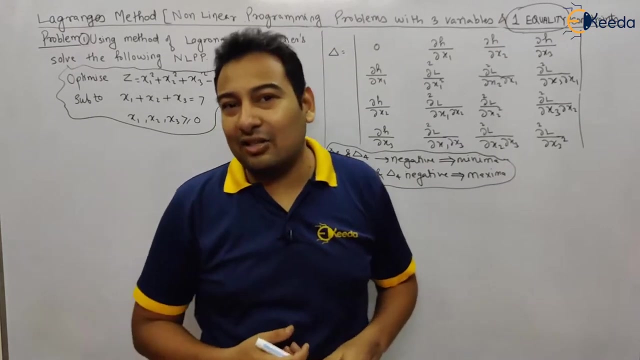 then it is maxima. again. you need to remember this condition that we'll discuss later. what is delta 3, what is delta 4, and so on. so let us start without wasting time. the procedure is exactly same. this is just a bigger version of what we discussed in the last. 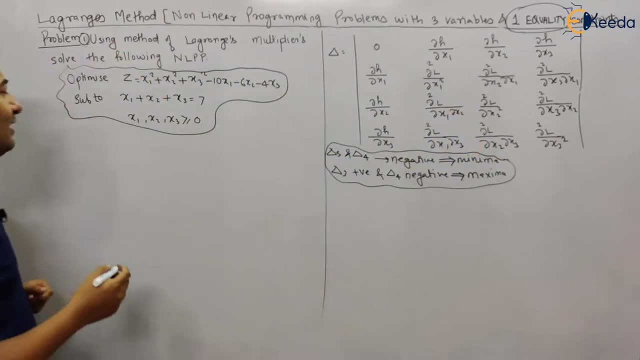 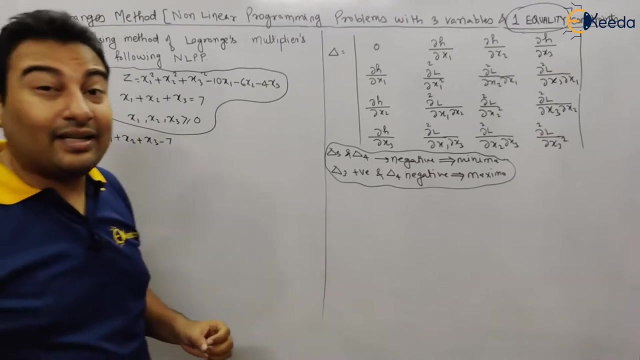 problem and the same story will be here. so first of all we're going to talk about the first of all, let us write it on h. h is the constraint, so here the constraint is 7. we're going to keep. take this side, here also we're going to find it out. take lambda, that is l, that. 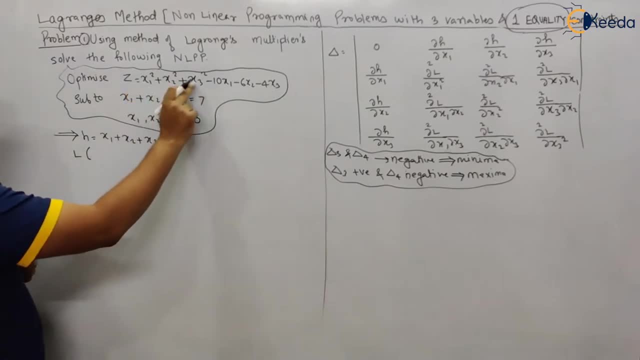 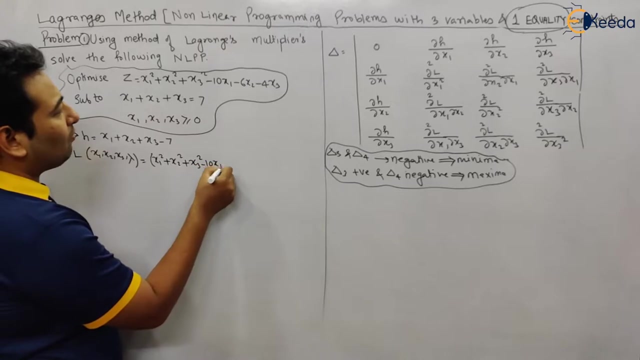 is your lagrangian multiplier. that will be a function of. there are three variables: x1, x2, x3 and lambda objective function. we're going to write it down first. similar procedure, exactly similar, just a bigger version of last problem, minus lambda times constraint. so what is the constraint here? this is your constraint. 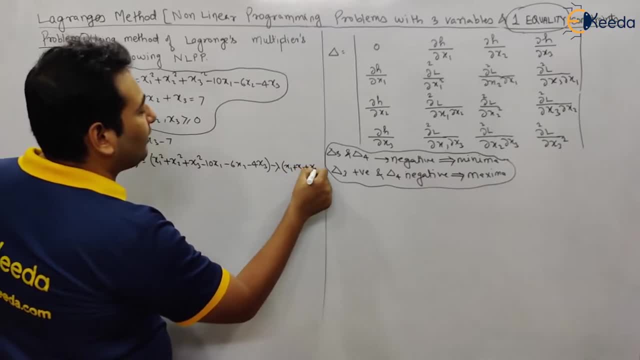 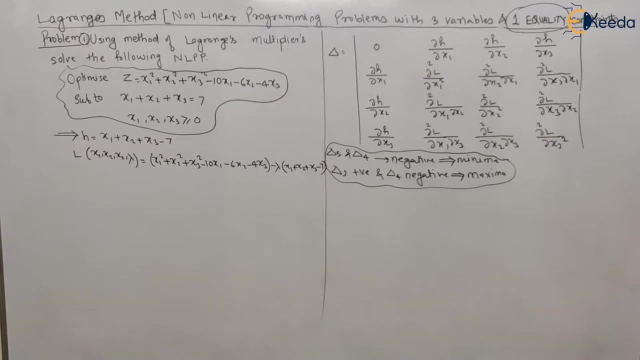 that is x1 plus x2 plus x3 minus 7. let us move on and let us discuss further this problem here. you know we can differentiate this l with respect to x1, x2, x3 and lambda, because this l is a function of x1, x2, x3 and lambda. so let us differentiate with respect to x1. 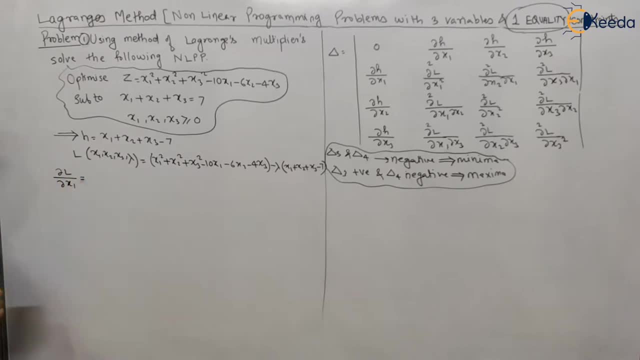 let us differentiate with respect to x1. so here it will be 2x1. what next? no x1. see here: minus 10. next this will be 0, 0 the. from this you'll get minus lambda. so this is your first next. now let us differentiate with respect to x2. this will be 2 x2. what next? 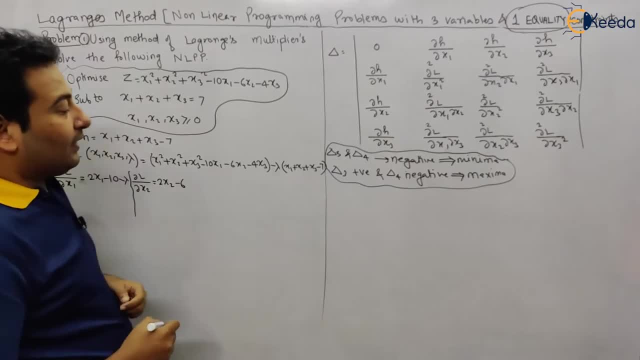 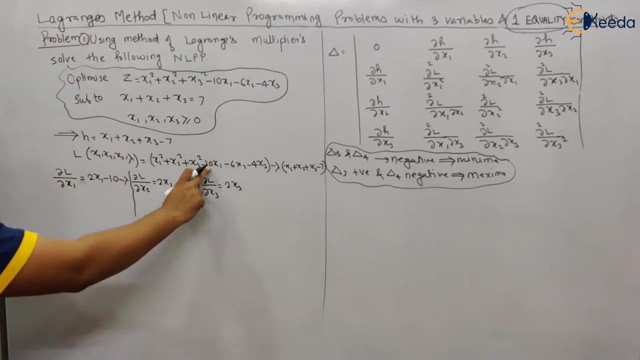 zero, zero. from this it will be minus six and from this it will be minus lambda. next, dou l upon dou x3. let us differentiate with respect to x3. so this is 2x3. next, 0, 0. here it is minus 4 and if you open it will be minus lambda. and last, 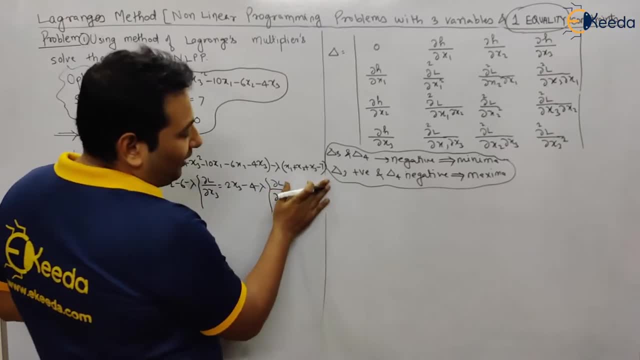 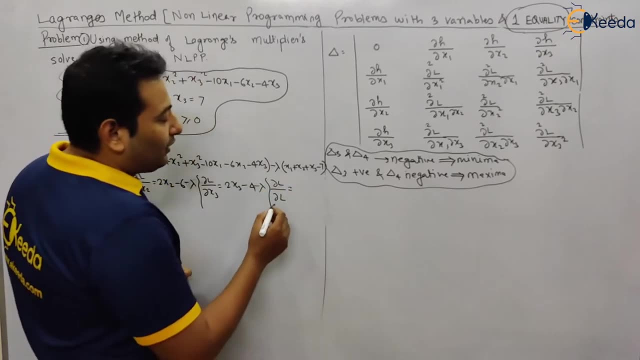 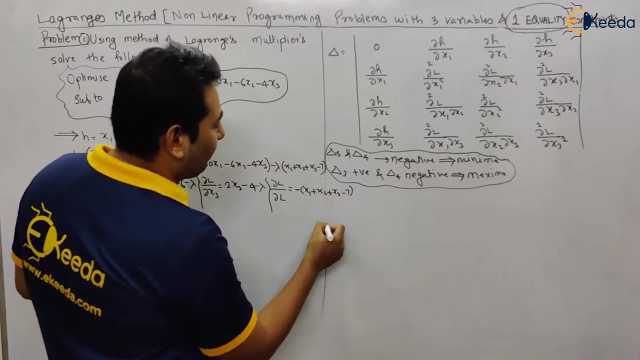 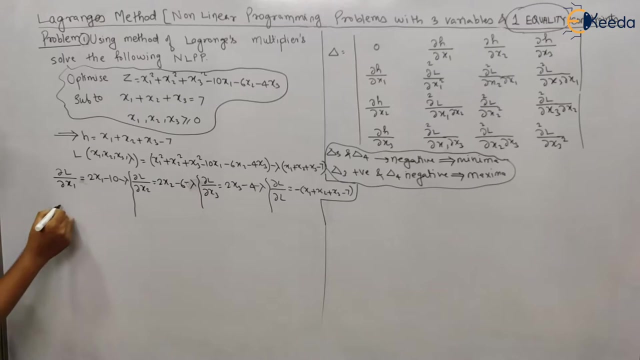 dou l upon dou lambda. we're going to differentiate with respect to lambda. so, with respect to lambda, obviously, all this is constant 0. we'll be left with the this minus x1 plus x2 plus x3 minus 7. so this is dou l upon dou lambda. what next? we need to equate all this equation to 0. 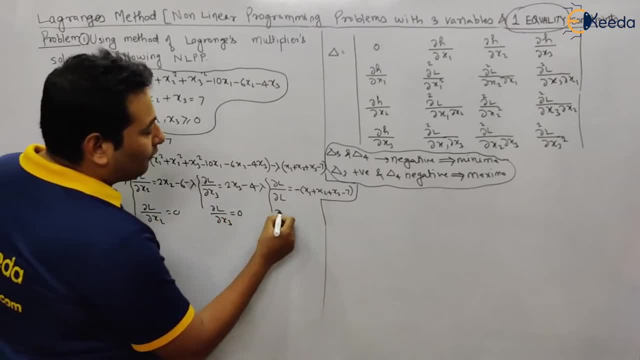 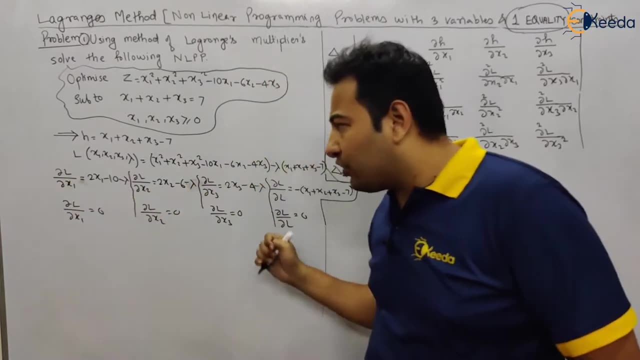 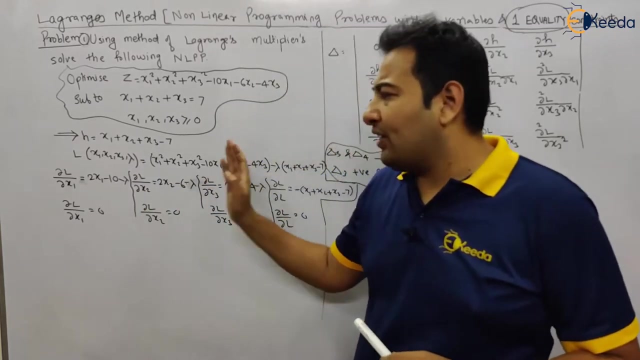 to get the value of, to get the value of x1, x2, x3 and lambda. in the last problem we equated to 0 and we got the value of x1, x2 and lambda. here there is one more addition of a variable that is x3. so therefore we need to find out x1, x2, x3 and lambda. but the simple story was in the last. 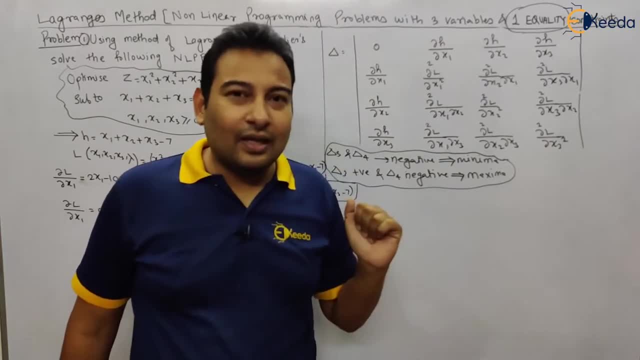 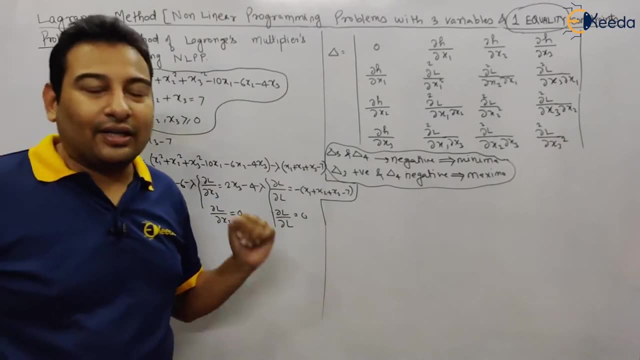 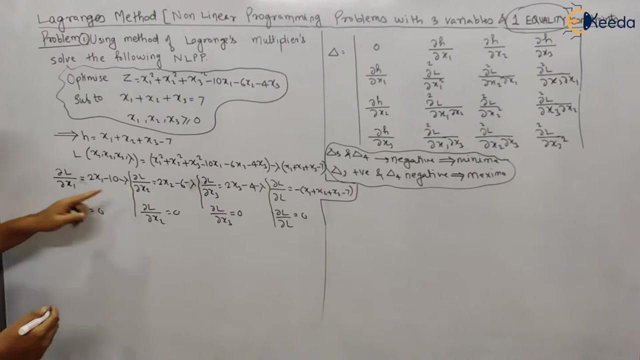 problem. there were only two, three variables, x1, x2, lambda. therefore we solved by using calculator. but there are four equations. it cannot be solved in calculator. you have to solve manually. so bit a tedious job, but we have to do it. dou l upon dou x1, that means this is equal to 0. 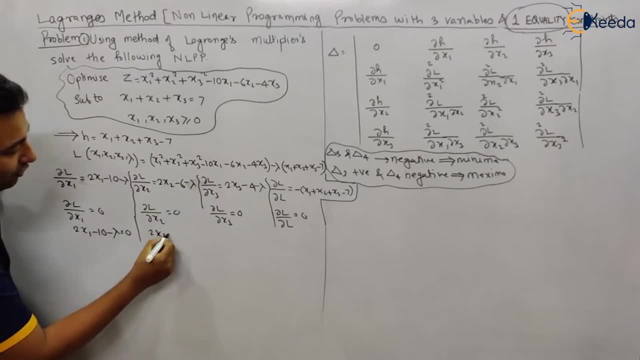 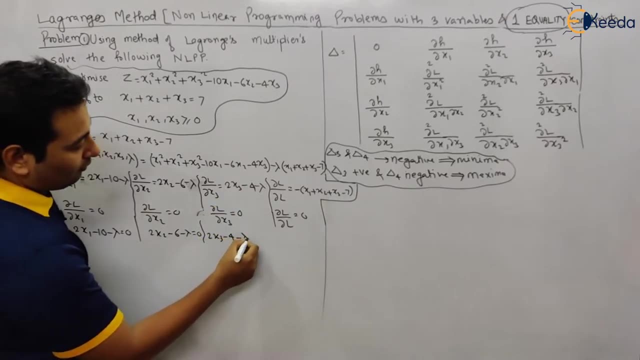 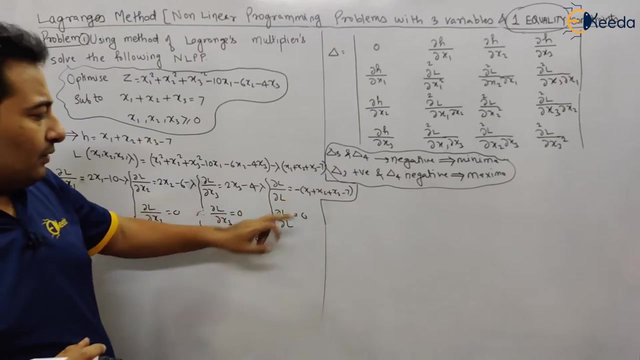 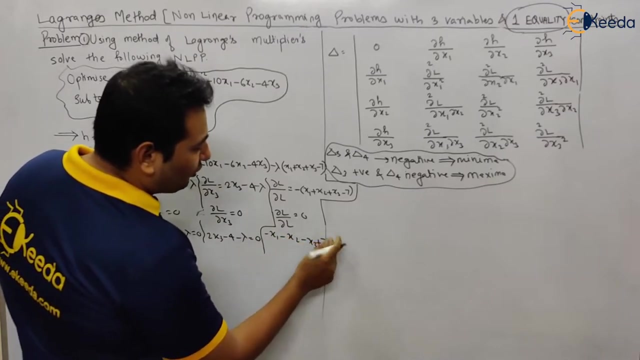 what next? this is equal to 0. 2 x 2 minus 6, minus lambda, equal to 0. what next? this is equivalent to 0. what next last? this is equal to 0. so, uh, let me write it down in this way. so if you, if you open this, minus x1, minus x2, minus x3 plus 7, equal to 0, simply. 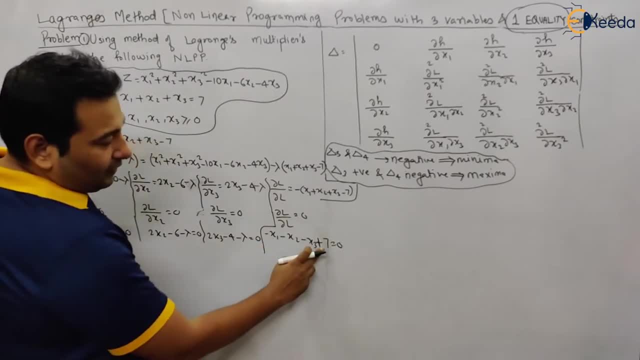 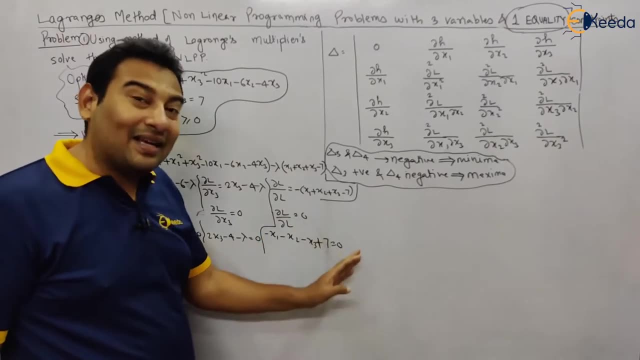 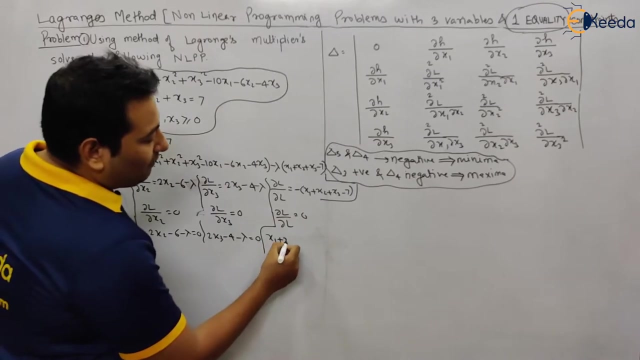 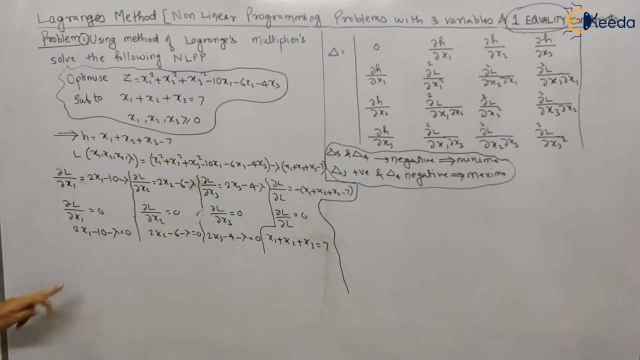 in short, you can write down this equation as see: if you take plus 7 that side, that will become minus 7. so this is minus x1 minus x2, minus x3, that's at minus 7. multiply throughout by minus. ultimately you will get a x1 plus x2 plus x3 equal to 7.. what next? we need to solve these four equations to get the. 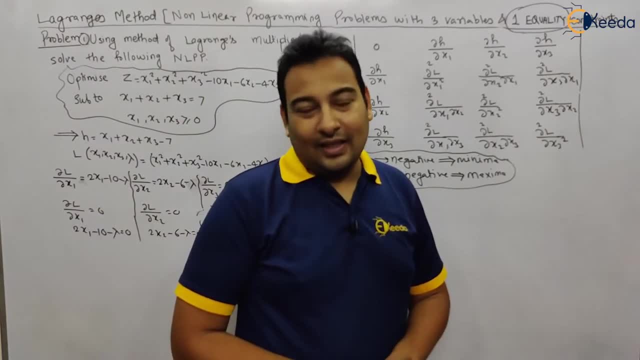 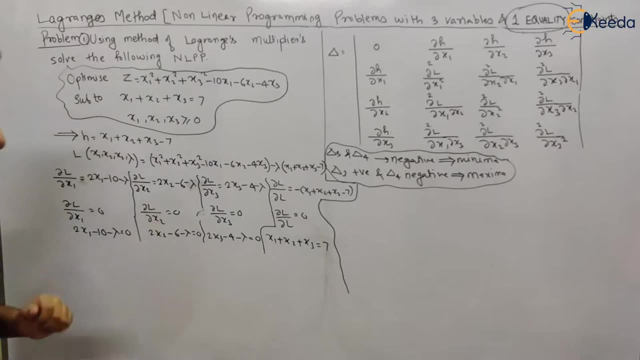 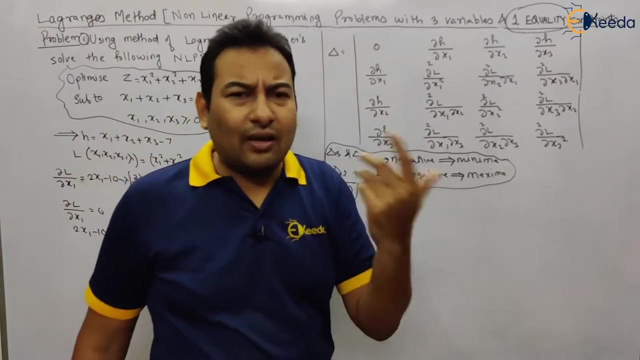 value of x1, x2, x3 and lambda. there are four equations. therefore we cannot solve in calculator, we have to solve manually. so let us do it now. there are few new calculators which allows solving four equation in calculator. if you have that calcul calculator you can solve by using uh. 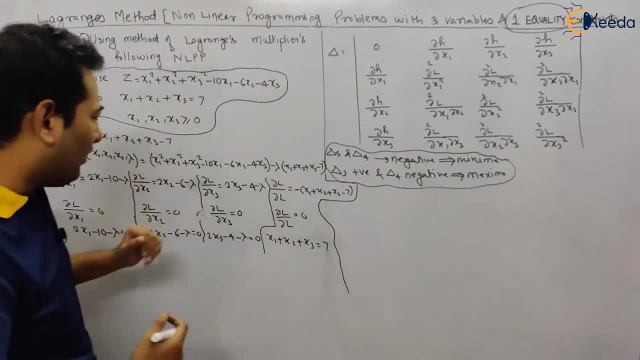 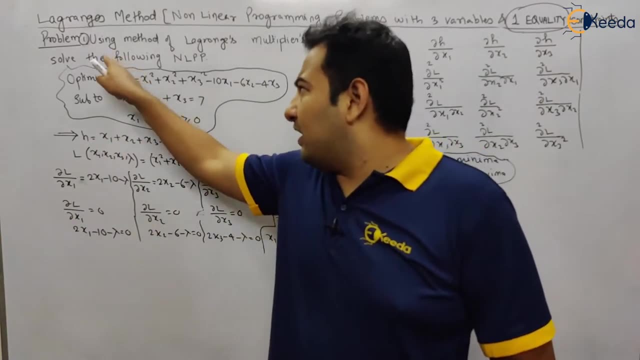 called celsius, but uh, i assume we don't have that calculator. therefore we're gonna solve it manually. so, and yes, the pattern: how to solve this four equation in this particular type. after that we'll be discussing one more example. in all the example, the pattern will be same. 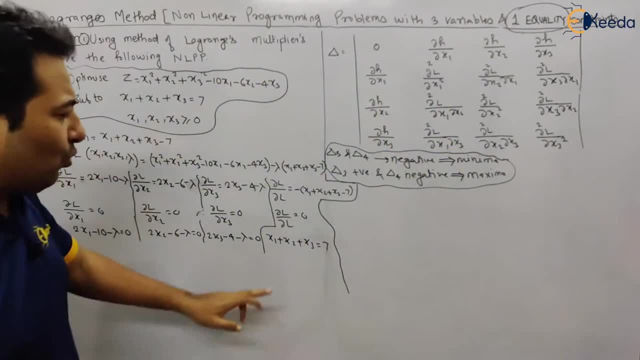 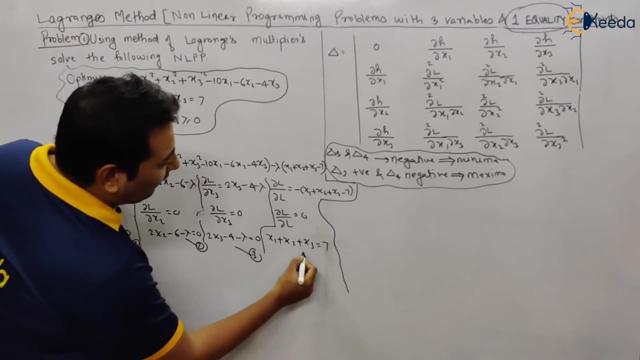 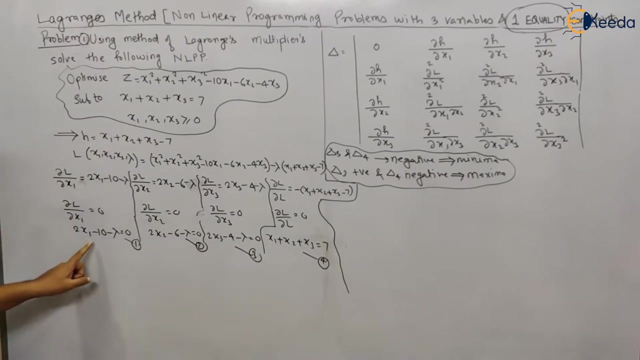 similar pattern to solve this equation. and see here the pattern is what? look at this equation. here we have x1, x2, x3. let us name it as one, two, three and four, 1 x 2 and x 3. if you add 1, 2 and 3, see, if you add 1, 2 and 3, you will get 2 x 1, 2 x 2, 2 x 3. let's add. 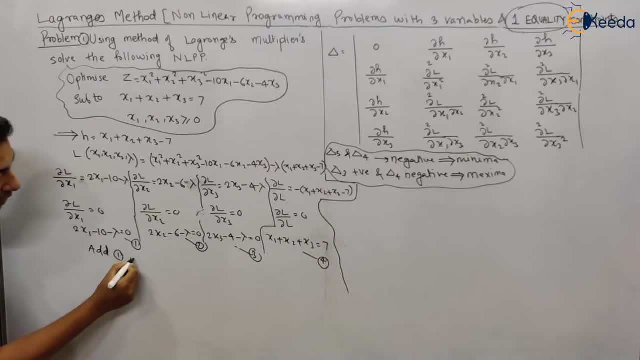 first of all, let us add, then we'll see 1, 2 and 3. if you add, you will get 2 x 1 from this. you will get 2 x 2 from this. you will get 2 x 3 from this. what else? from this, you will get minus 10, minus. 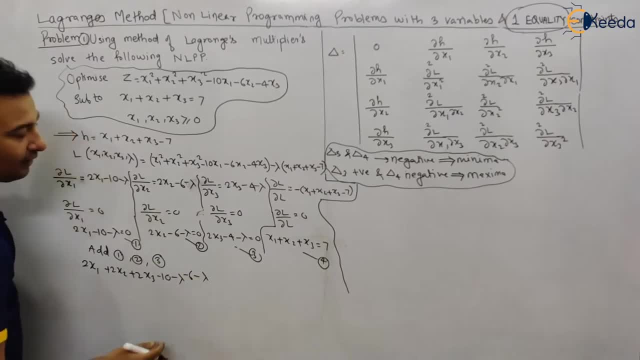 lambda from this, we'll get minus 6. minus lambda: from this, we'll get minus 4, minus lambda, equal to 0. let's take two common from this: x1 plus x2 plus x3 minus 10, 6 and 4. that is minus 20. 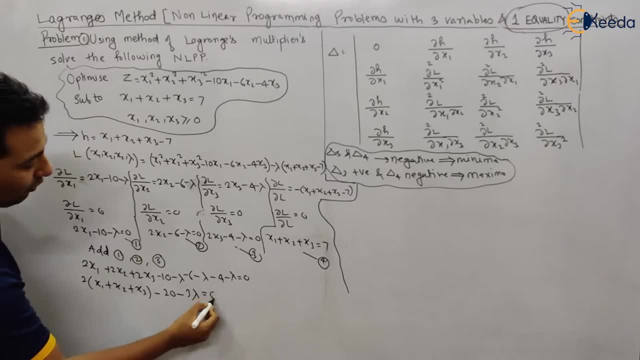 minus lambda minus lambda minus 3 lambda, equal to 0. now check from equation number 4: x1 plus x2 plus x3 equal to 7. so let us put here: 7: x1 plus x2 plus x3 is what 7? this is from. 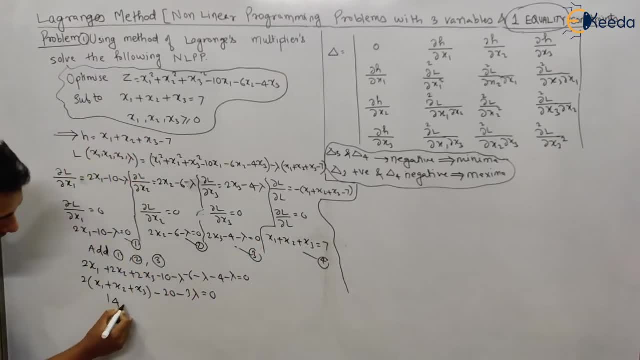 equation number 4. if you put 7, this will become 14 minus 20 minus 3, lambda equal to 0. so if you simplify, 14 minus 20 will be minus 6. therefore, lambda is equal to minus 2. we got the value of lambda that is minus 2. 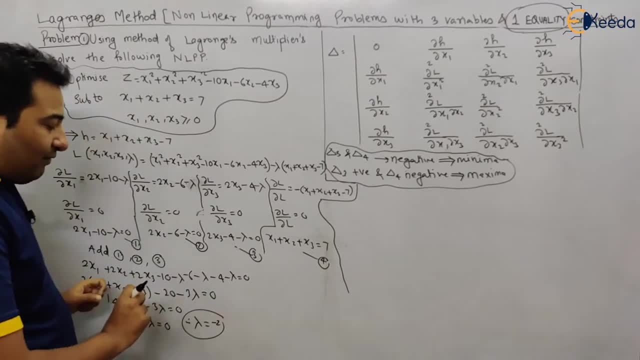 what next see? we evaluated one variable. now what we can do, we can simply put this lambda in equation number 1, 2 and 3. if we put in equation number 1 lambda, that is minus 2, we'll get the value of x1. if we put lambda is equal to minus 2 in equation number, 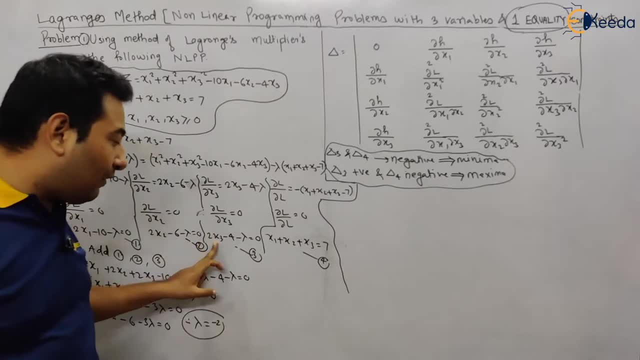 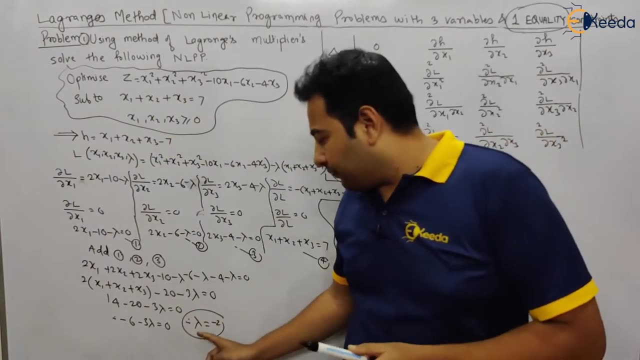 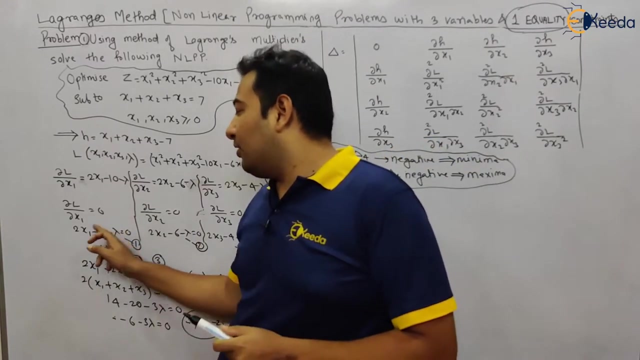 2, we'll get the value of x2. if we put here, we'll get the value of x3, and that's it. so that is that are the values that are required here. after putting the value of lambda in equation number 1, 2 and 3, we're directly getting the values if you put lambda here. 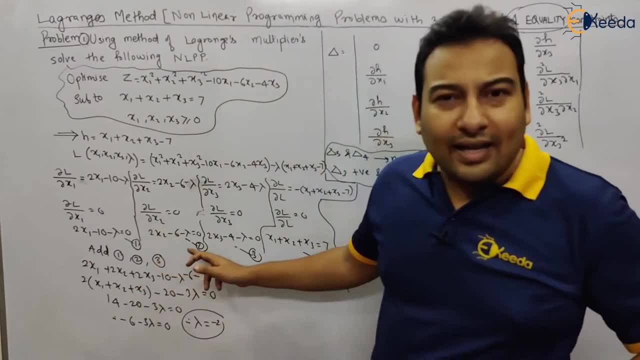 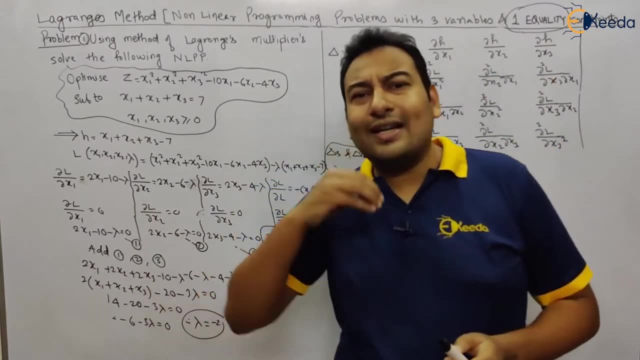 directly get the value of x1. if you put here will get directly get the value of x2 and if you put here you will get the value directly of x3. but it is not. it is not necessary. there may be a situation: if you put lambda here, you will get. 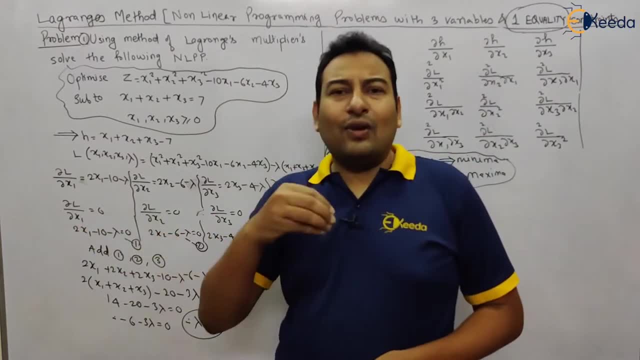 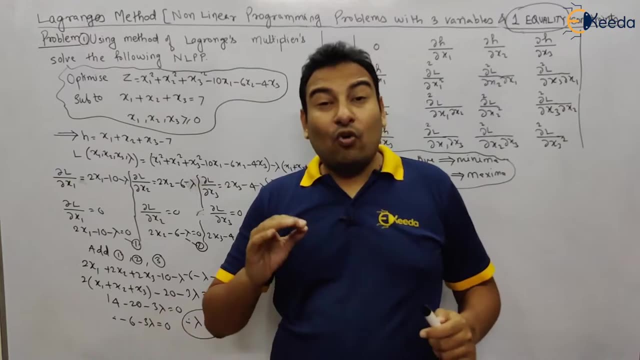 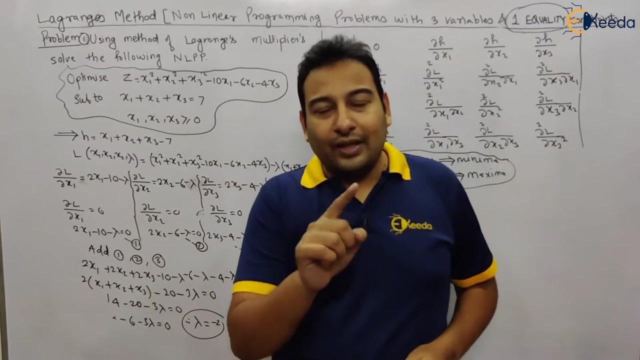 three equations and if you get three equation you can solve by using calculator to get the solution. see what was the problem? the problem was here we are getting four equations and we cannot solve. but once we get the solution of one value, that value you can put in the remaining equations and you 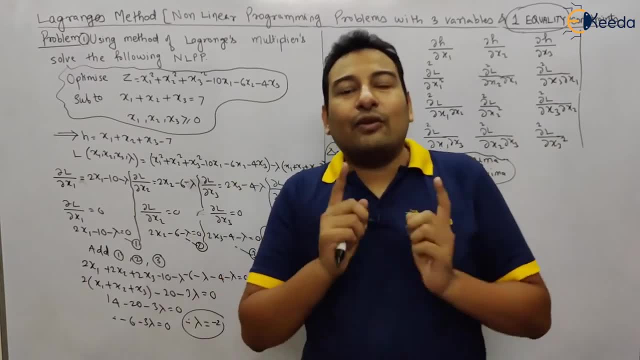 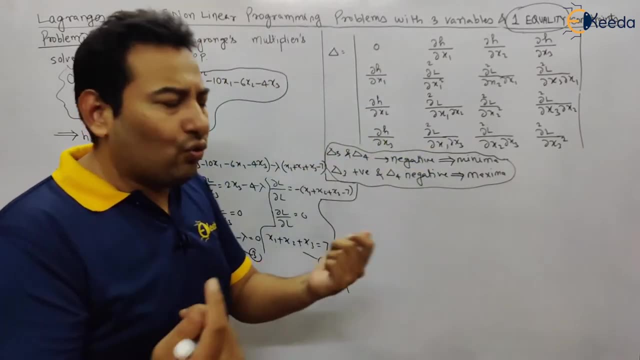 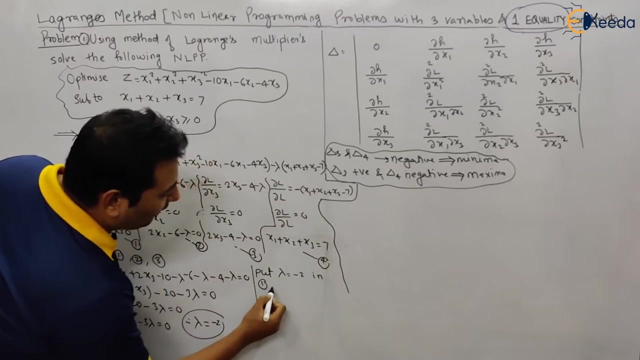 can convert four equation into three equations, and after that you can put this equation in calculator to get the solution. so this is a manual work, so you can manage the way you want. so let us put lambda equal to minus 2 in 1, 2 and. 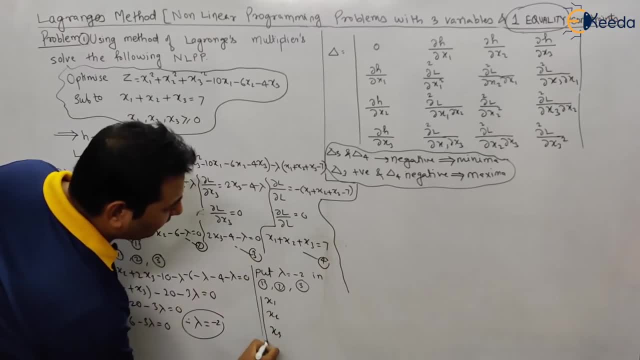 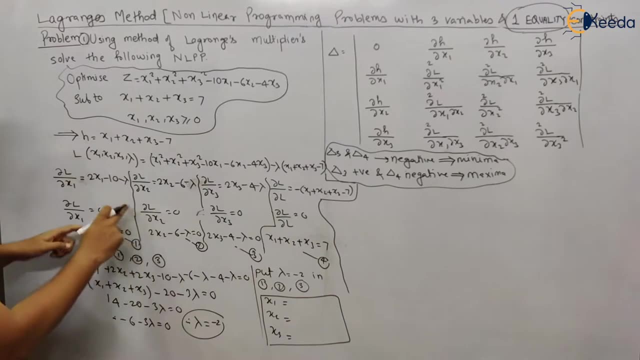 3. if you put, you will get X 1, X 2 & X 3. so let us get the values X 1 equal to. let us put lambda equal to minus 2 here, so this is minus 2 minus minus plus, so that will become plus 2 minus 10. plus 2 means minus 8, so that side will go and will. 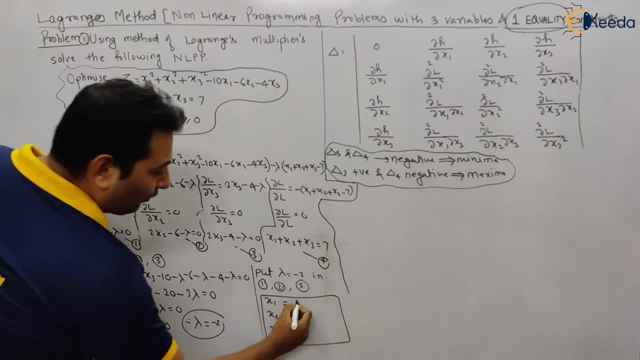 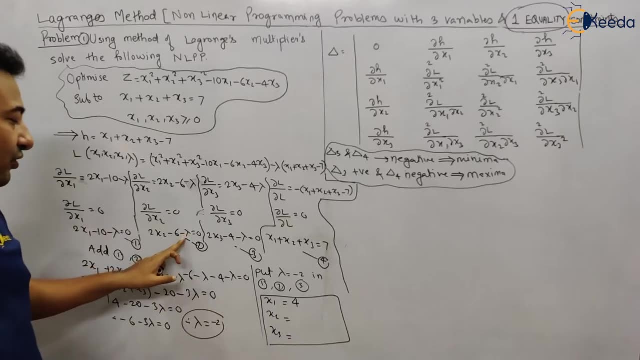 become plus eight. two X 1 is equal to 8. X 1 is equal to four. you solve by writing. you will get the result: lambda is minus 2. then again it is 2 minus 6. plus 2 is minus 4. will go to that side, will become plus 4, that is. 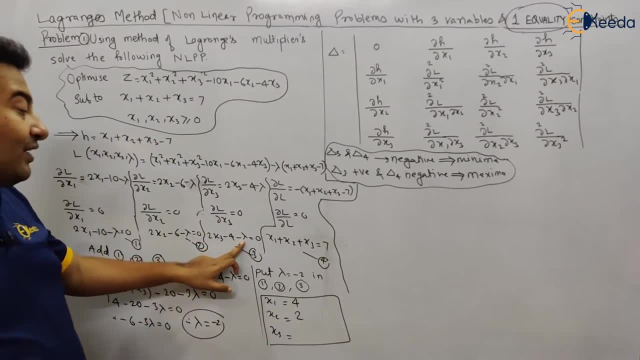 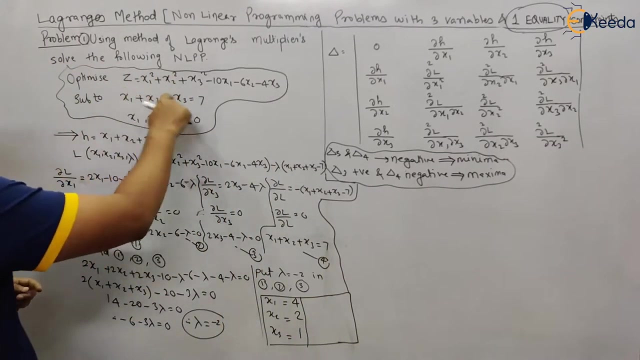 2 answer. and if you put lambda is equal to minus 2 here, that is 2 minus 2, 1. so these are the values of x1, x2 and x3. so we got the solution. if i'm going to put this x1, x2 and x3 in my z, i'm going 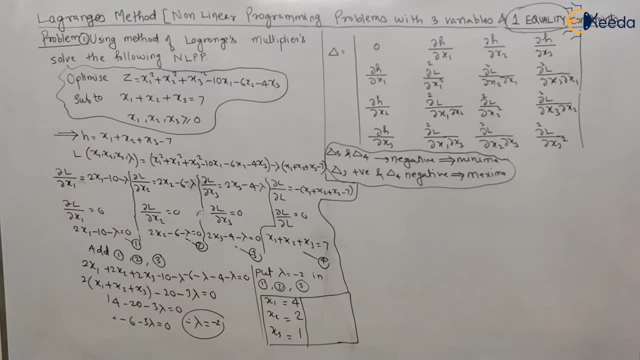 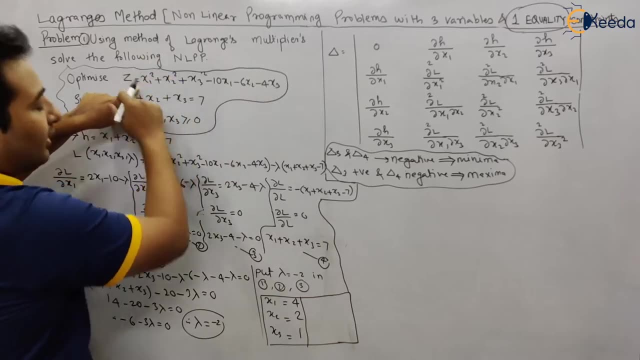 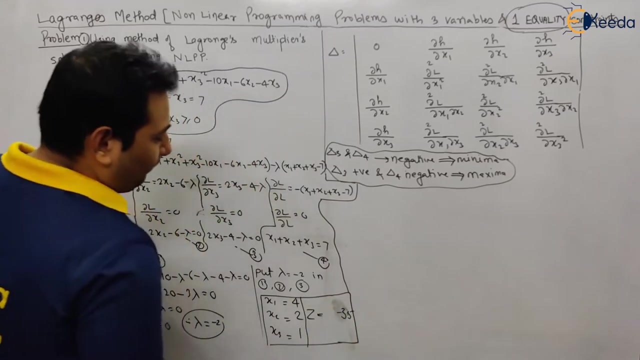 to get the solution for this particular problem and the solution that i'm getting. after putting this values 4, 2, 1 in this particular equation put here, the value of z will be minus 35. you can use calculator to check. put x1, x2 and x3 here and you'll get the value of z as minus 35. 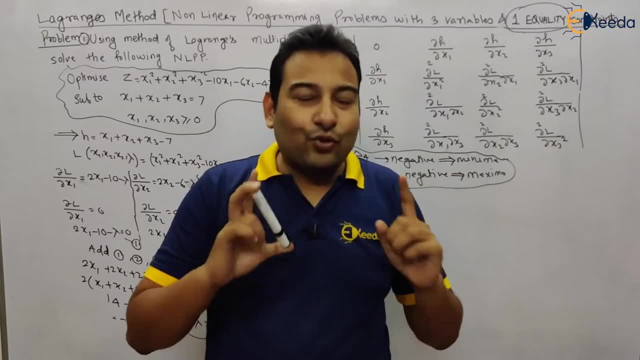 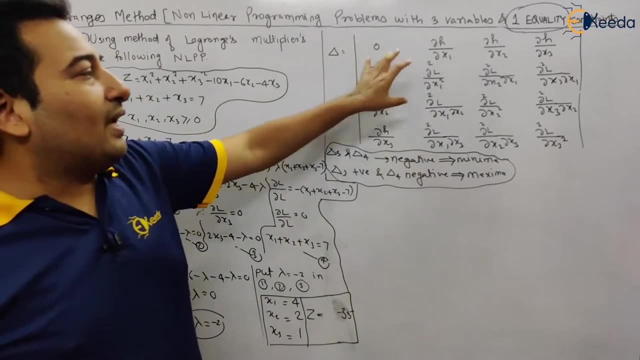 but what is the problem? the only problem is to check whether this value is a maximum value or a minimum value. you can use calculator to check whether this value is a maximum value or a minimum value. for finding that, we need to take help of this. so let us find it out. delta here. 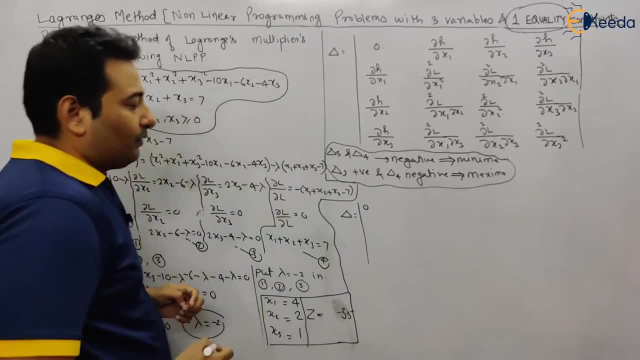 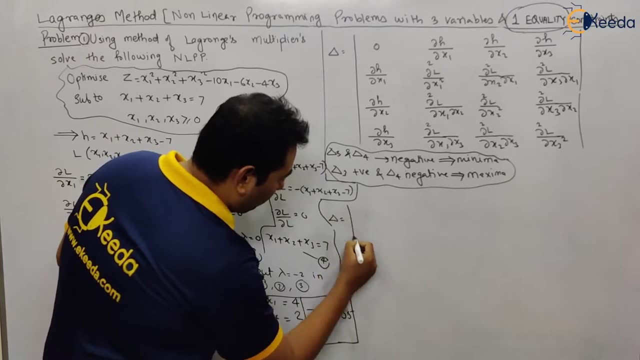 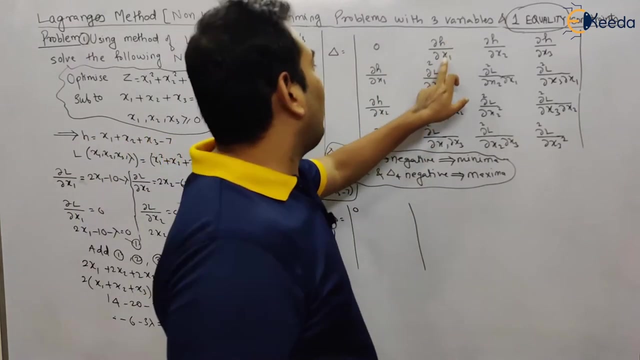 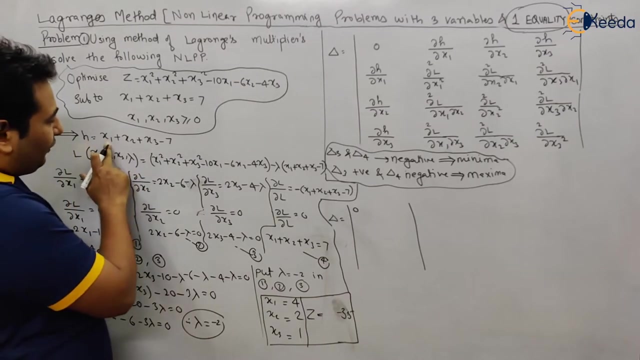 this is 0. next dou h upon dou x1. let us save some space. 0 next dou h upon dou x1. that means this h i'm going to differentiate with respect to x1. then it is 1 because with respect to x1 this is a constant term. its derivative is 0, again with respect to x2. 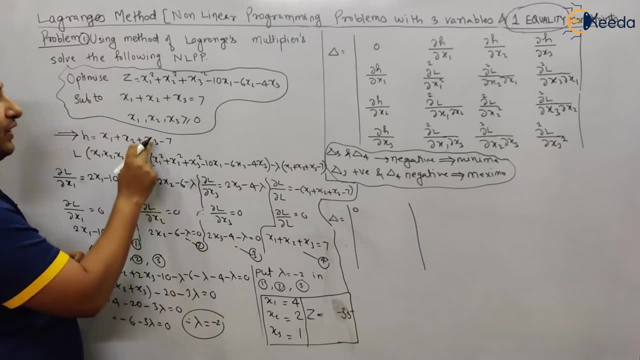 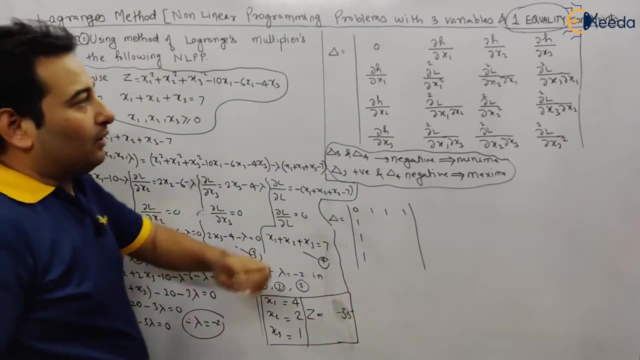 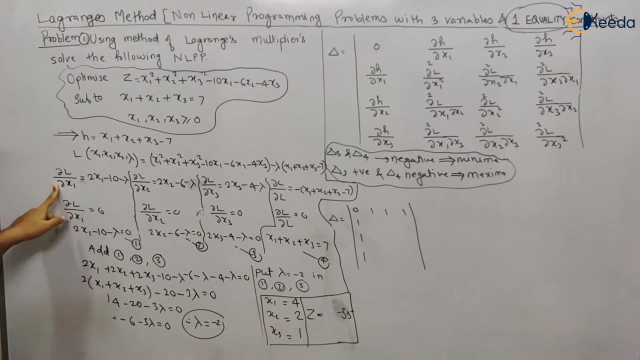 it's 1 because its derivative is 0. again with respect to x3: derivative 1. so basically, here it will be. next, dou square l upon dou x1 square. this is your dou l upon dou x1. we are going to differentiate one more time with respect to x1. so this is 2. derivative will be 0. so here it is. 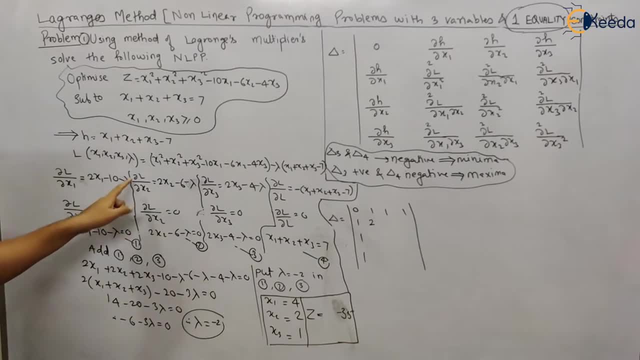 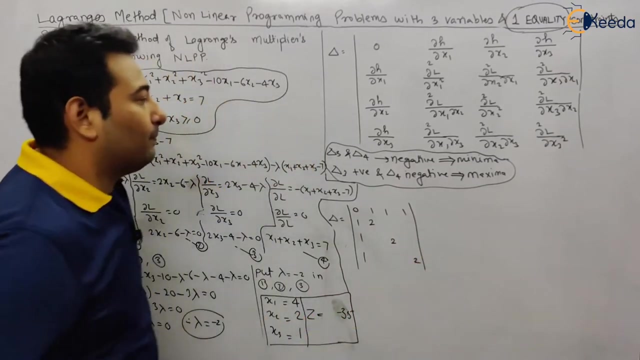 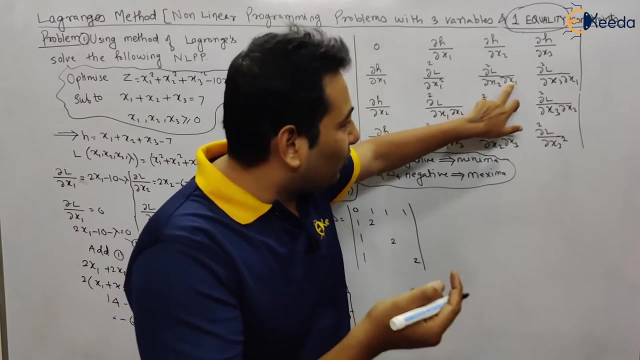 2. next, dou square l upon dou x2 square will be 2 and this dou square l upon dou x3 square you're going to differentiate with respect to x3. its derivative will be 2, here it will be 0. next, now see, these two terms are same: dou l upon dou x2. differentiate with respect to x1 or dou l upon. 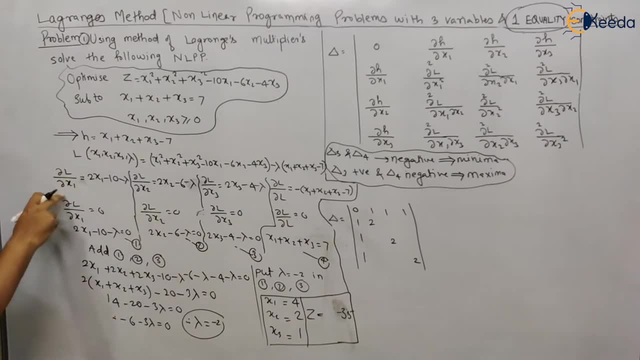 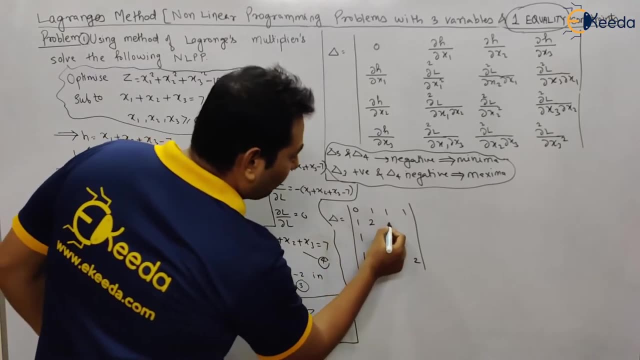 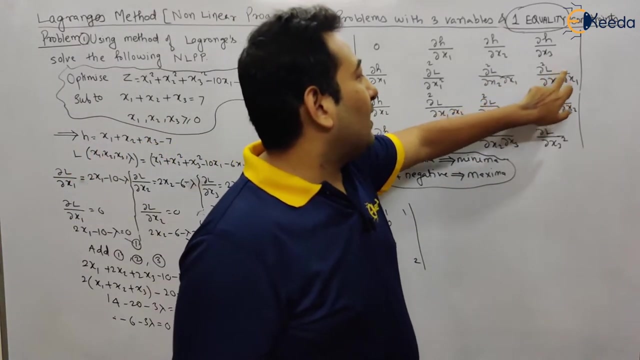 x1. differentiate with respect to x2. one and the same thing. this is dou l upon dou x1, let us differentiate with respect to x2. so when we differentiate with respect to x2- this is your constant term- its derivative will be 0. so here, and these two terms are the same. next, dou square l. 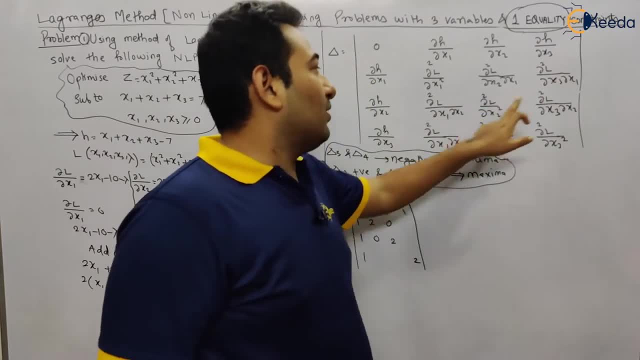 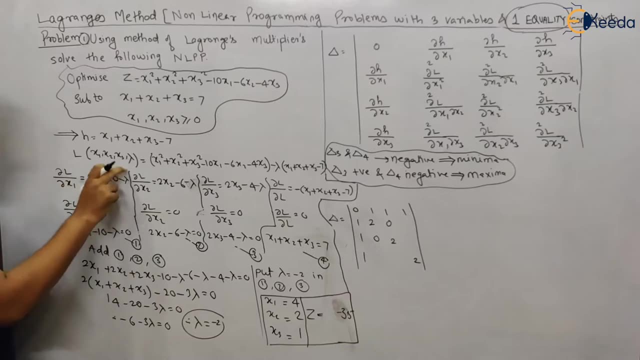 upon dou x3, x1- see here. both the terms are the same. so x1 we're going to differentiate with respect to x3. so if you differentiate x1 with x3, that means this result with x3- obviously it's a constant derivative- will be 0. what next last? 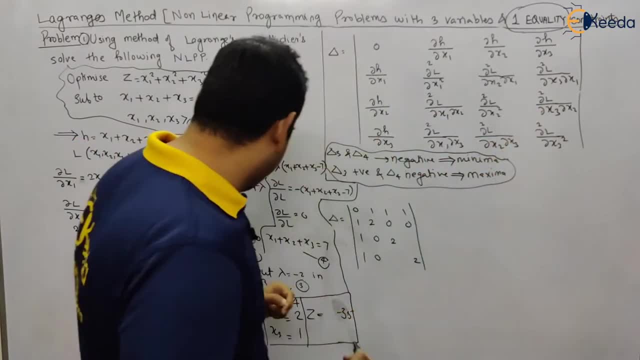 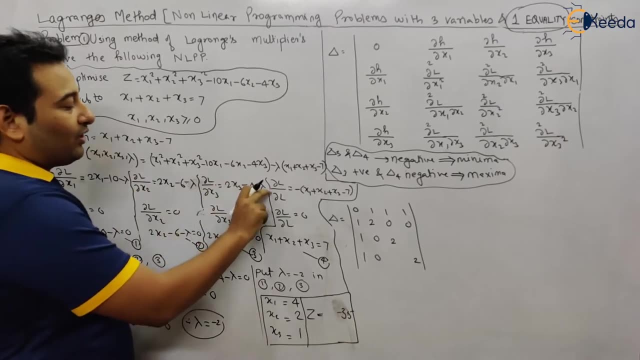 these two: x3 with x2, x3 with x2 or x2 with x3, whatever you do see here, with respect to x3: 0. with respect to x2: 0, whatever you do, it's a 0. so we got the value of delta. now what is the condition? 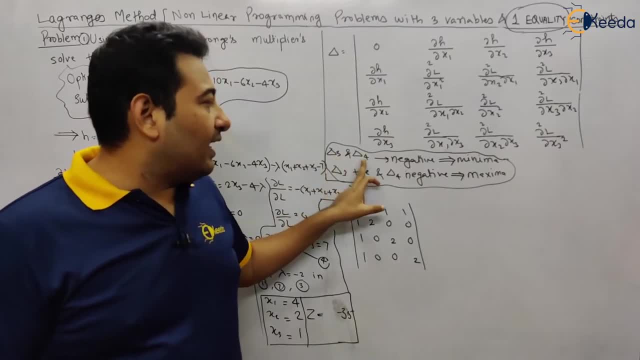 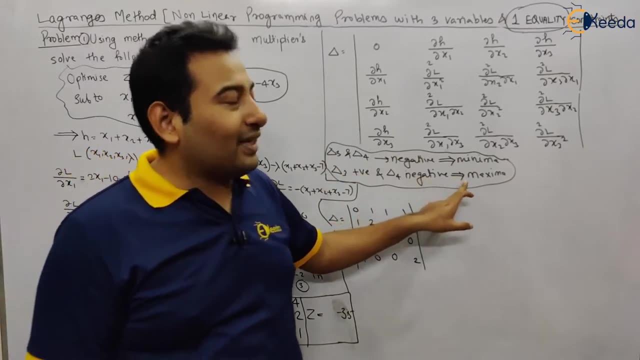 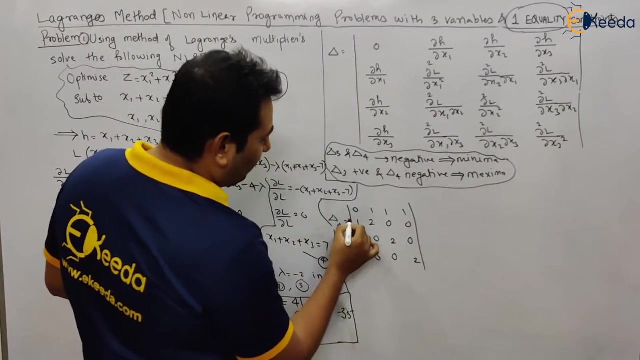 the condition is: delta 3 and delta 4. both are negative, then it is a minima, and if delta 3 is positive and delta 4 is negative, then it is a maxima. what does this mean? very simple, see, this is your delta 4. simply, delta 4 means 4 cross 4. and what is delta 3? 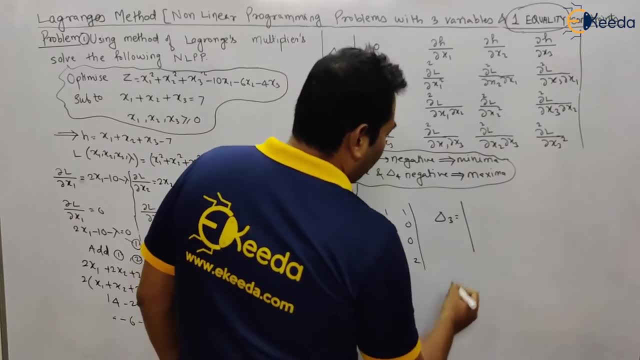 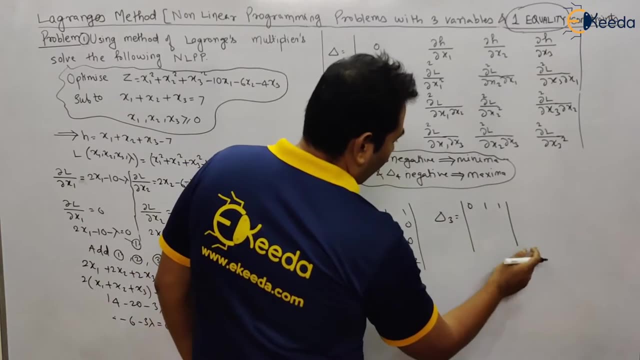 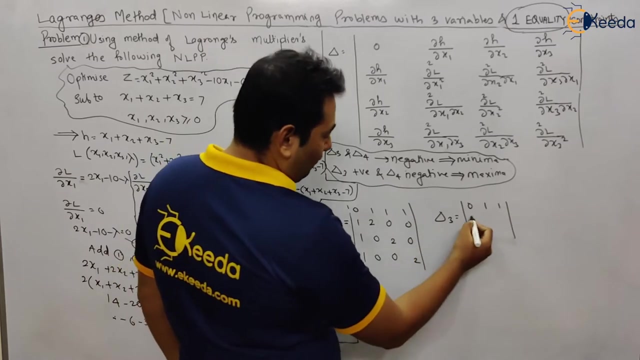 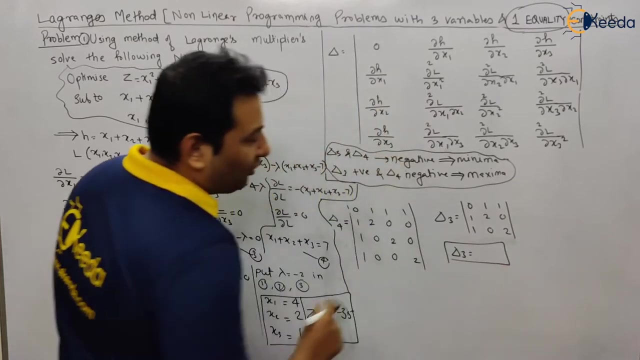 delta 3 means 3 cross 3. so 3 cross 3 means first 3 rows and 3 columns. see here: this is delta 3: first, 3 rows and 3 columns. 3 cross 3. you can directly manage in calculator and you can directly get the answer of delta 3. 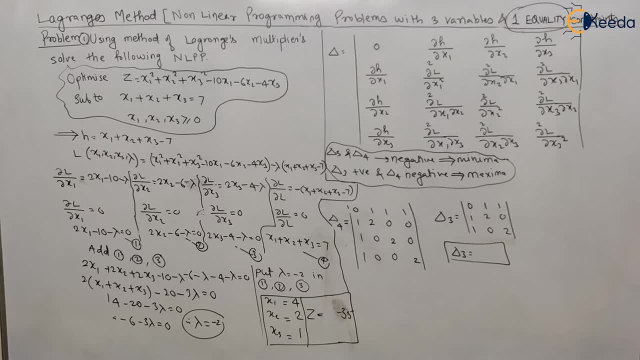 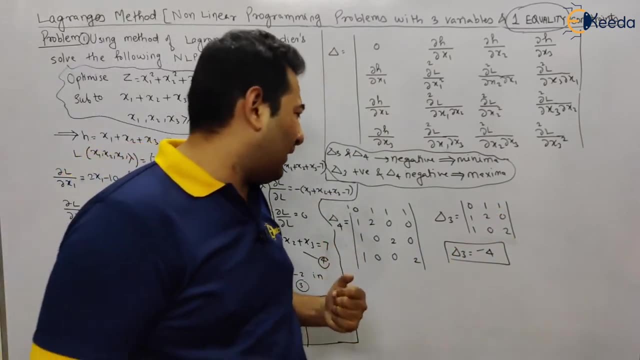 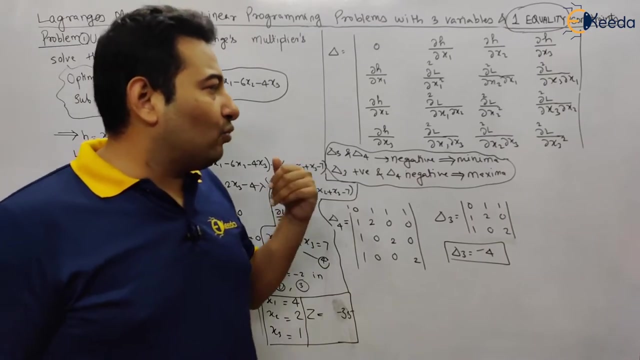 delta 3. answer that we getting is minus 4. so here it is minus 4 directly: 3 cross 3. you can directly manage in calculator or you know how to solve right. what about this now? delta 4: 4 cross 4. you have to do it manually. let me write it down: delta 4. 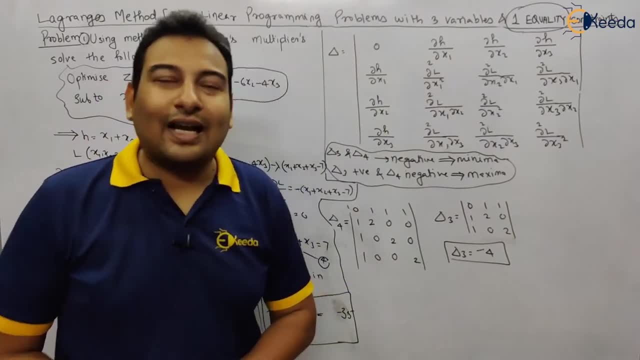 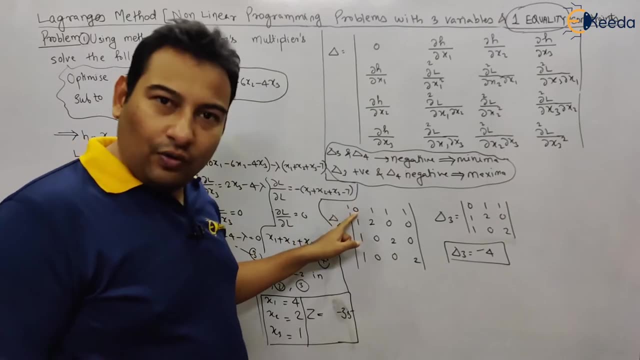 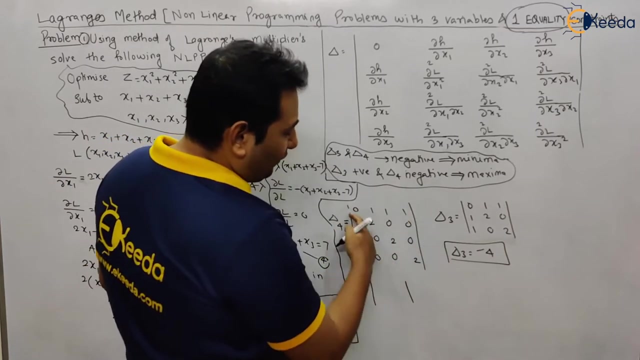 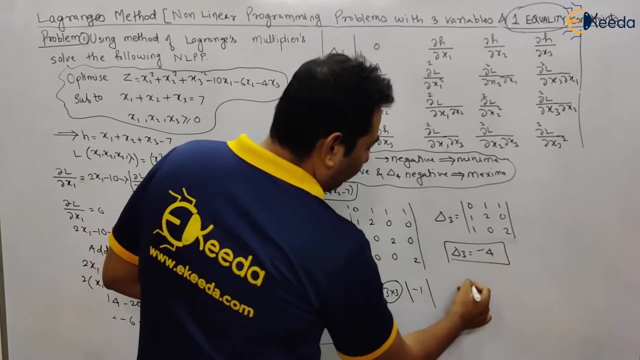 here, see delta 4. you have to do it manually, so for that purpose, how to solve? see delta 4 means what? 0 and after that a 3 cross 3. leave this column and this, leave this row, and you will be left with this 3 cross 3 here. then minus 1, minus 1. leave this column and this row, and after that i. 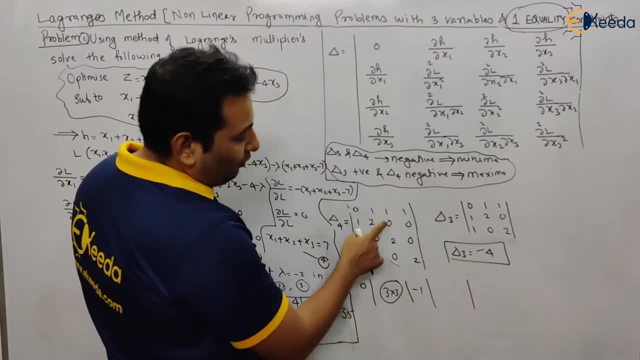 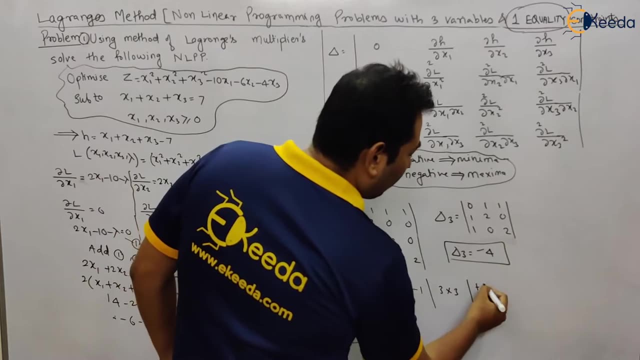 will be left with this 3 cross 3. that is 1, 1, 1, 0, 2, 0, 0, 0, 2. there will be 3 cross 3 alternate plus minus, so 0 minus 1, then it is plus 1. i'm going to leave this column, this row, so i'll be left with. 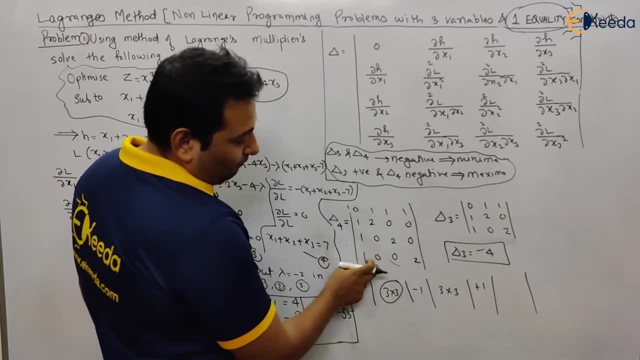 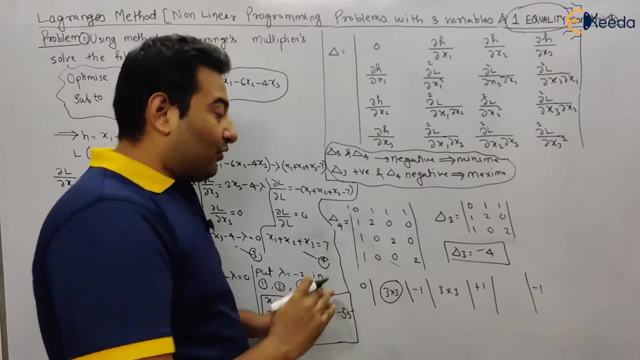 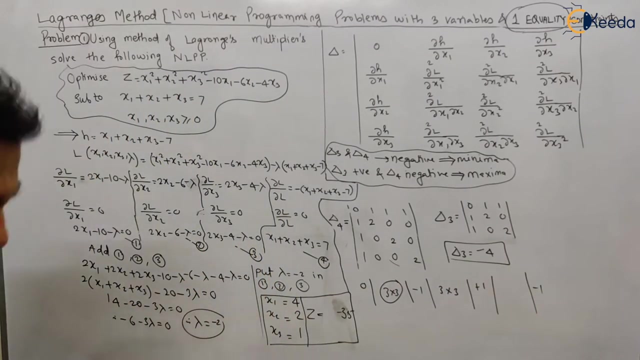 these two and this, and finally minus 1 for this, leave this column, this row, and i'll be left with this 3 cross 3. so and after that, you need to solve all this plus and minus to get the solution. so that will be a bit lengthy. you can easily, you can do it, but that will take some time. 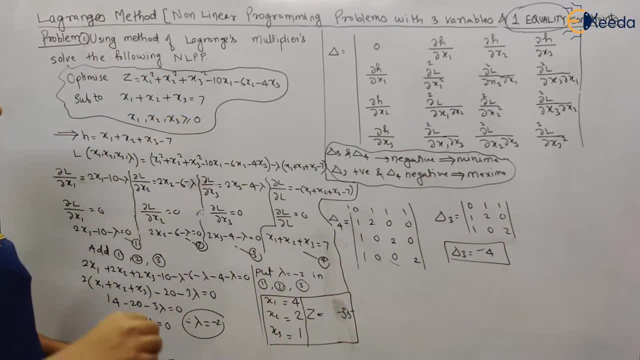 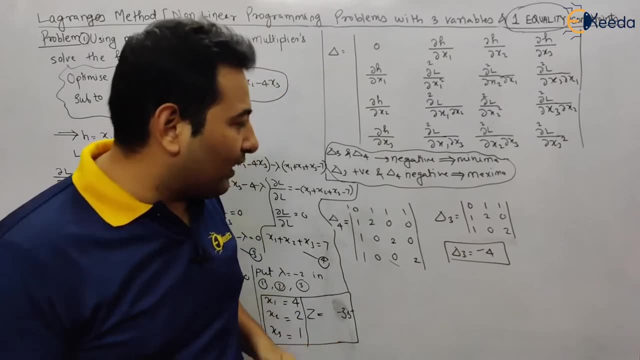 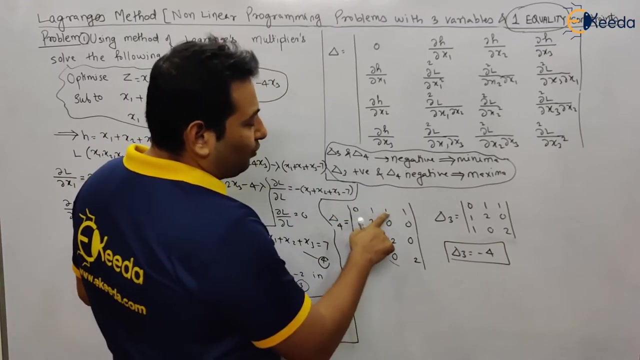 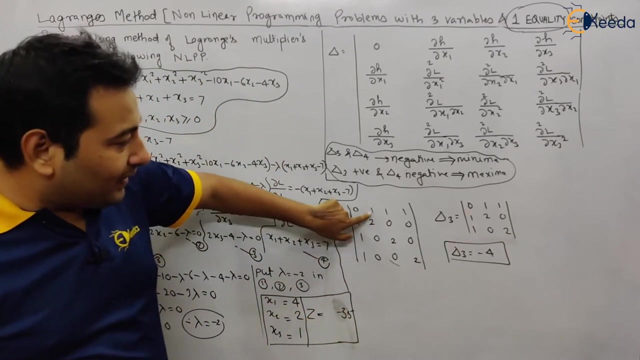 we can do it in a much simpler way. how? let us perform some column operations to get the solution. obviously, you can do it. this is your C2, C3 and C4. so what I am doing? C2, I am making this C2 and C3: 0 with the help of C4. 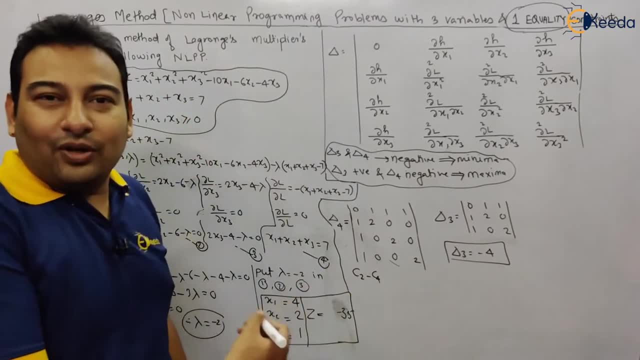 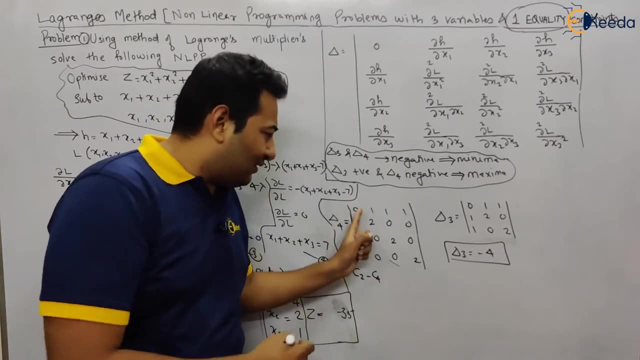 C2: 0 with the help of C4. I hope you are aware about these operations. if you are not comfortable with this operation, you can go ahead with the way that we just discussed this and this and just before this. whatever, I have given this idea to you. 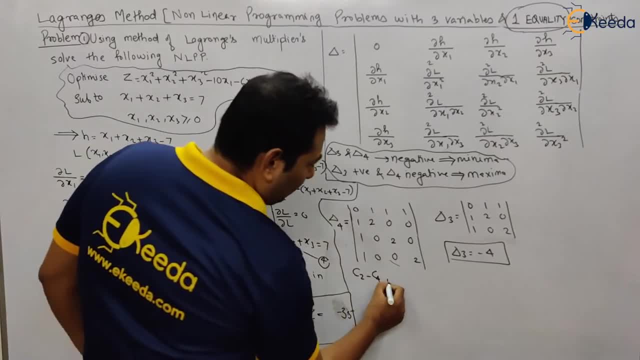 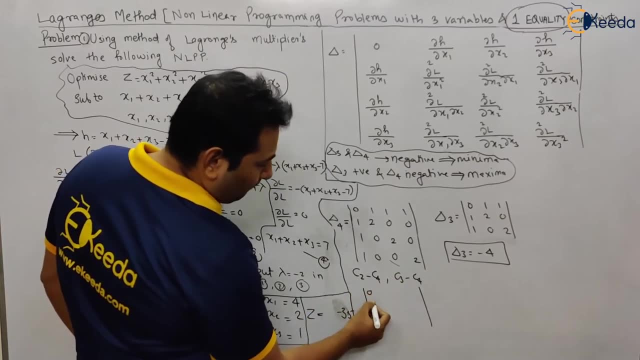 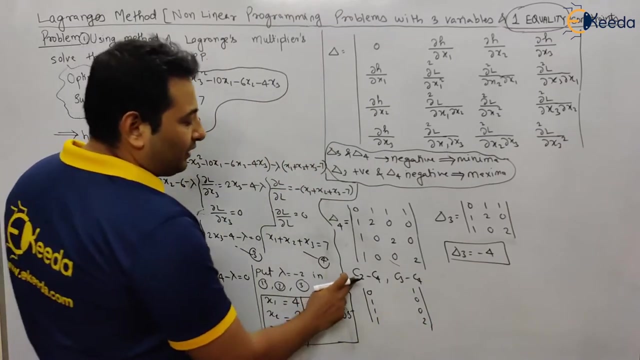 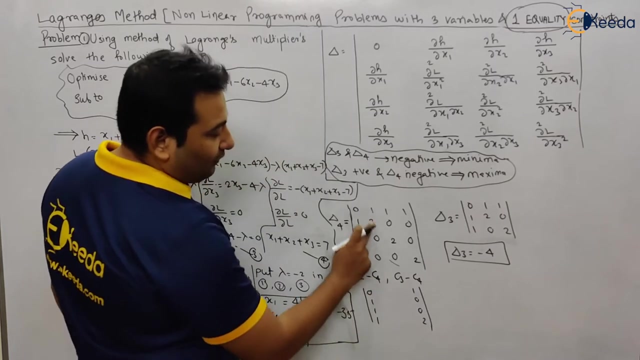 written here as a rough work that you can go ahead with that: c3 minus c4, c2 and c3 will change. c1 will remain same and c4 will remain same. what will happen? c2 minus c4. so basically from c2 we are subtracting c4, c2 minus c4, that is 1 minus 1, 0 and changes we're going to write down in c2. 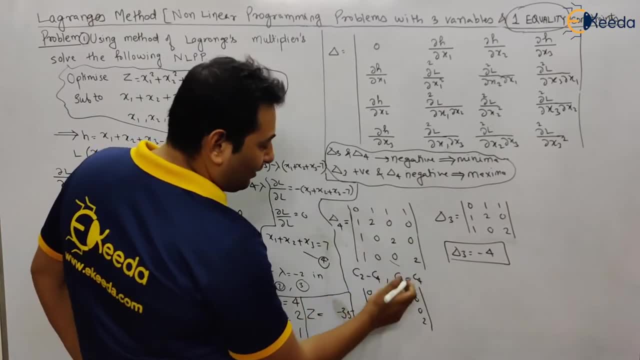 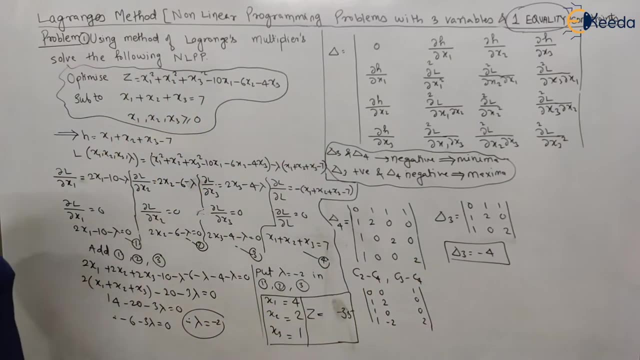 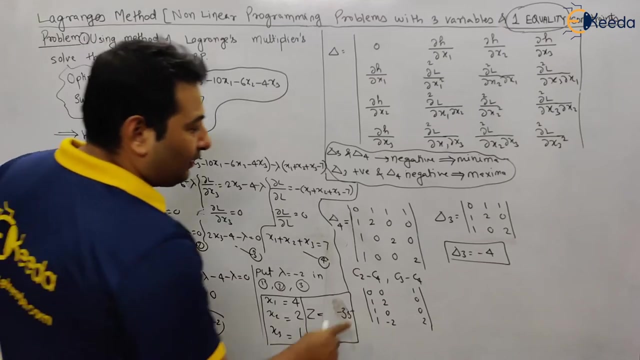 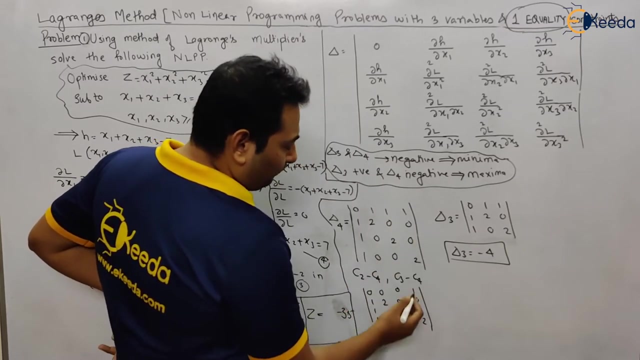 2 minus 0. 2. 0 minus 0. 0. 0 minus 2 is minus 2. c2 minus 4. c4. next up. next we're going to write it down: c3 minus c4 c. this is a c3 minus c4. 1 minus 1. 0. 0 minus 0. 0. 2 minus 0. 2. 0 minus 2 is minus 2. 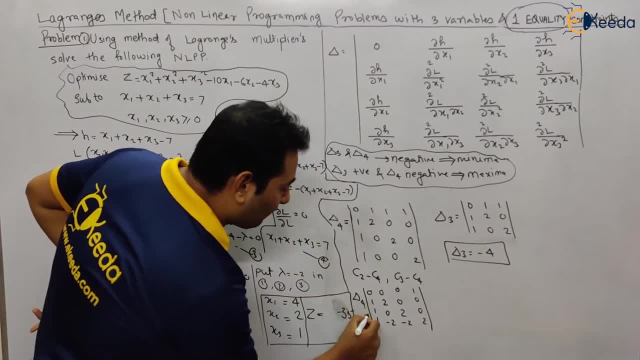 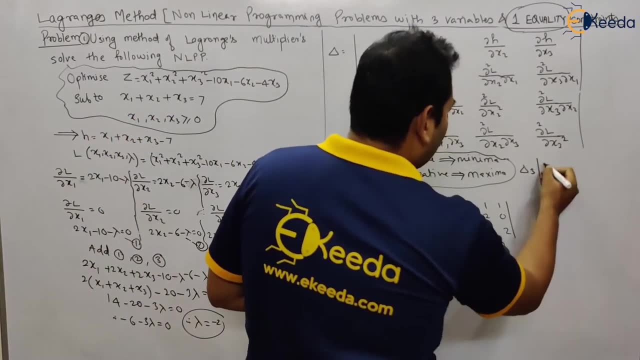 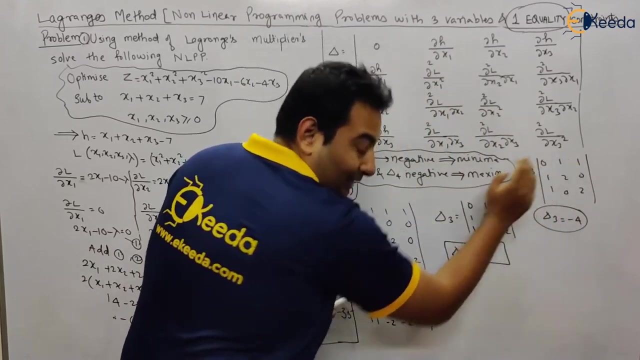 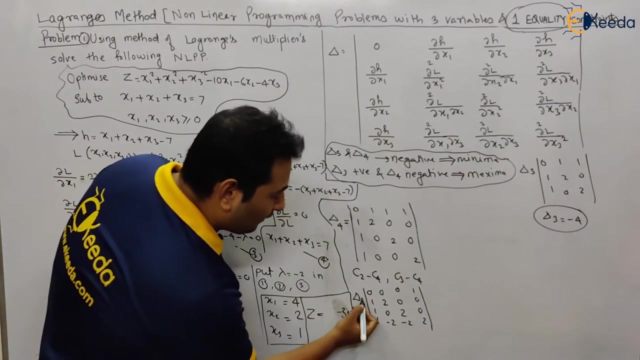 so this is your delta 4. can you please tell me what is the advantage? let us write it on delta 3 here, so just to save some space doing nothing. just shifted there so that i'll get some space to write. see, here, this is my delta 4. how to further simplify it? now it's very simple. 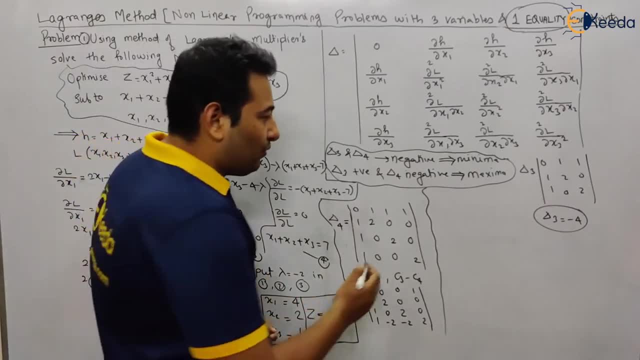 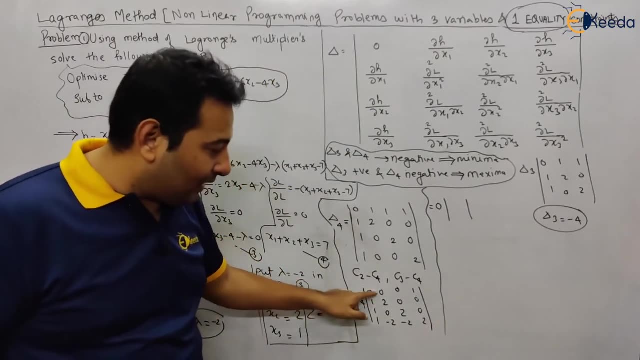 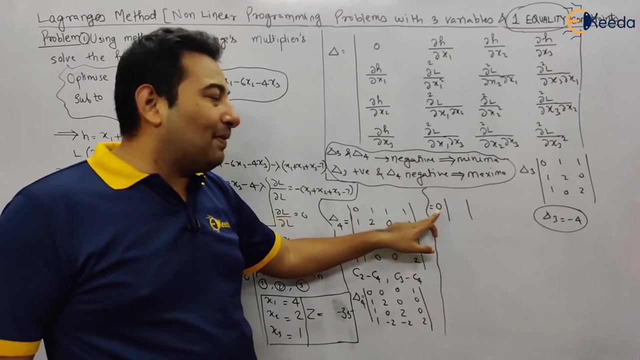 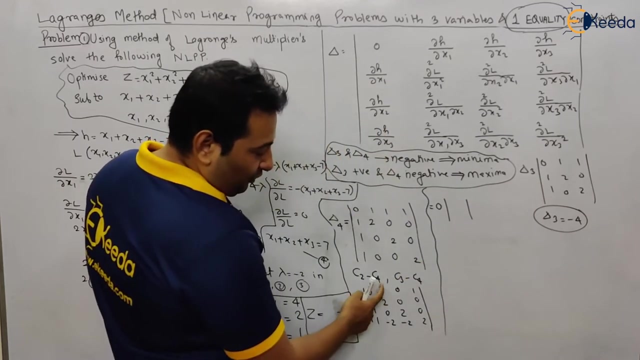 0 into cn. there will be a determinant here. this 0. leave this column and this row and write it down, this determinant. but whatever you write, if you multiply it by 0, that will be gone. that is 0 only, so no need to write again. again, we have 0, so 0. there will be a determinant. leave this column. 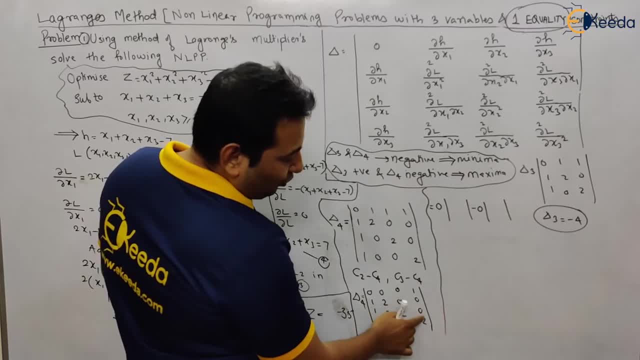 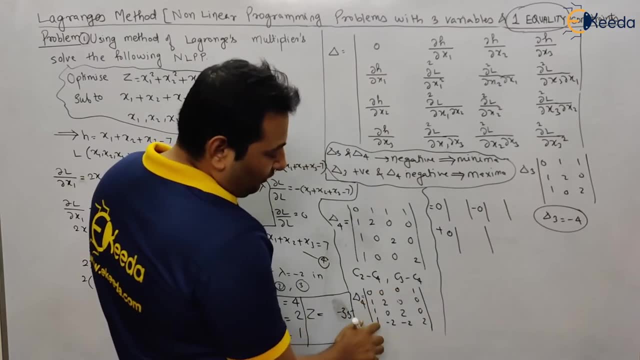 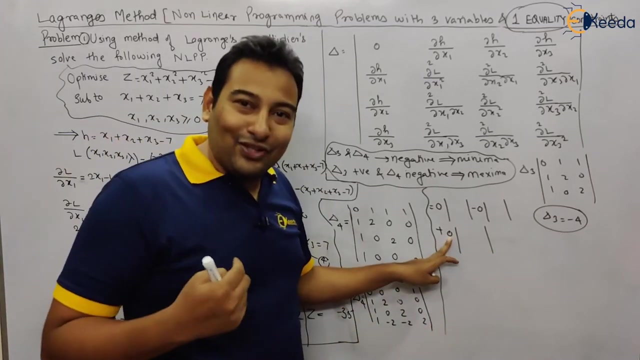 and this row. so triple one, zero two minus two, zero zero two will come here, so doesn't matter, leave it again. again, we have zero. leave this column and leave this row will be left with this, but that will also be gone, because it's multiplied with zero and it's alternate plus minus. first is positive. 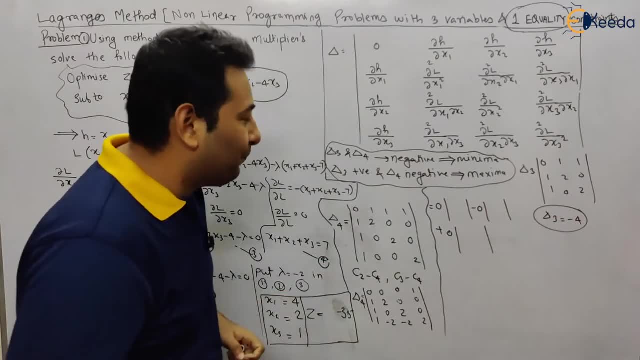 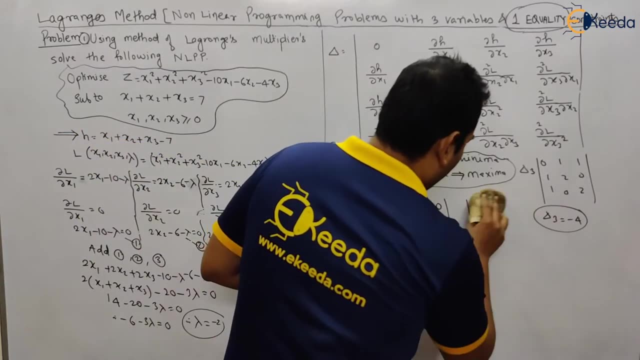 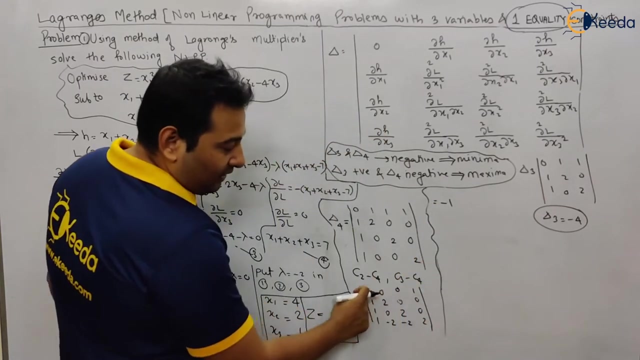 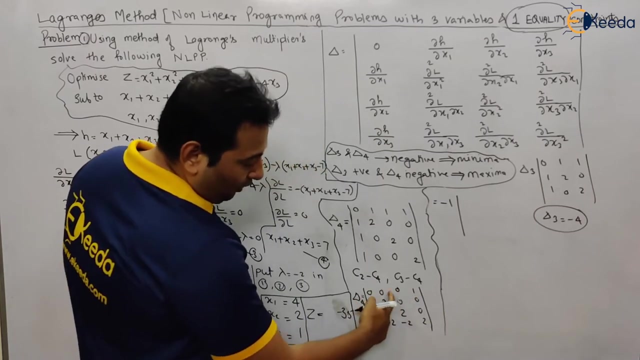 then negative, then positive and finally negative. so, in short, no need to write all these things. and will be left with the. will be left with the directly minus one, because rest everything, if you multiply by zero, it will be zero, only minus one into. leave this column and row and we left. 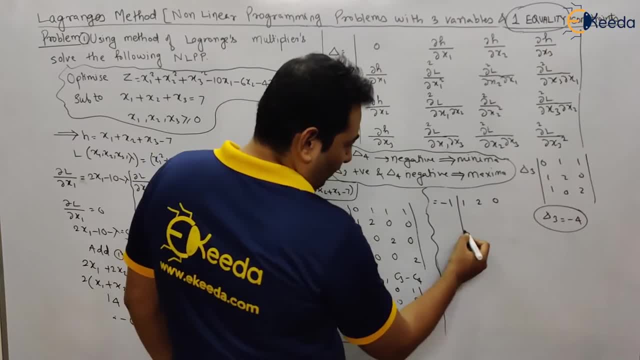 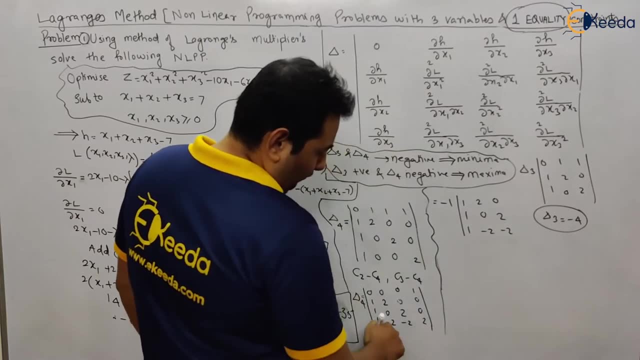 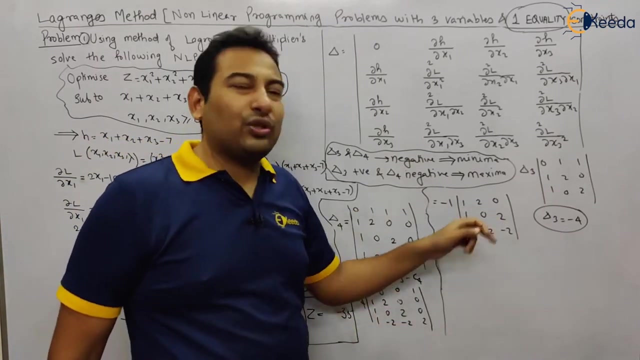 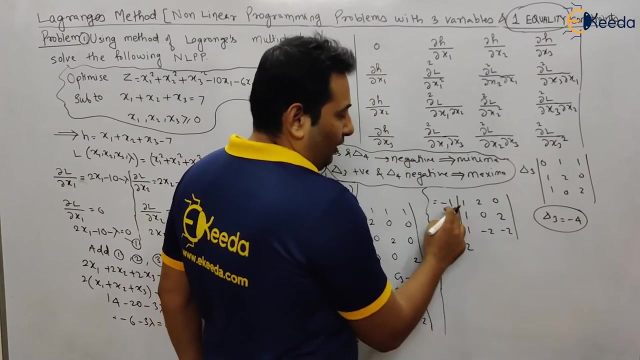 with this, that is, one, two zero one zero two and one minus two minus one minus two and two, one minus two and minus two. now we converted this four cross four into three cross three. three cross three. you can solve in calculator and if you do it you will get. the answer is twelve, and outside we have 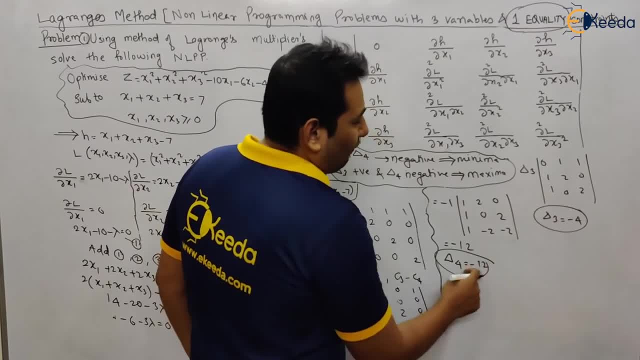 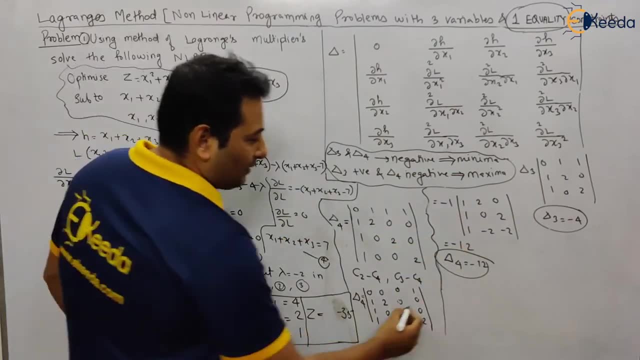 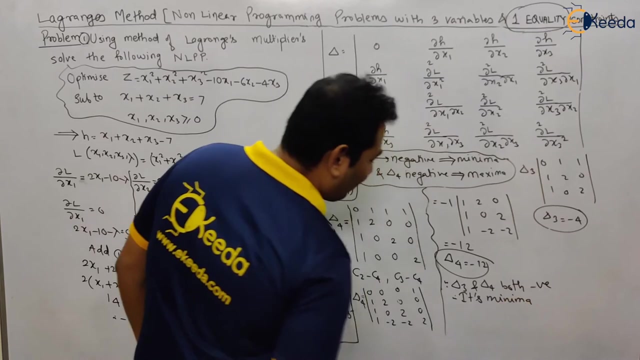 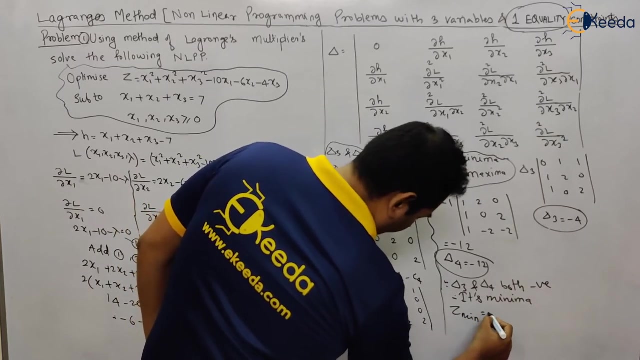 minus. so, in short, delta four is equal to minus twelve. see here both the negative values, delta three and delta four, both negative. what does this mean? minima, and what is the final answer? z, so it it's actually z minimum. so the final answer is suppose it would be: delta three would be positive and delta four would be negative. 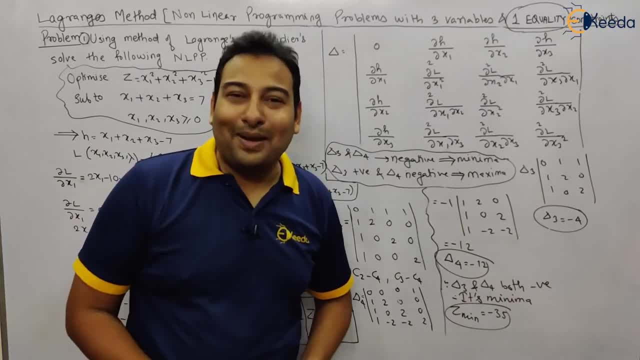 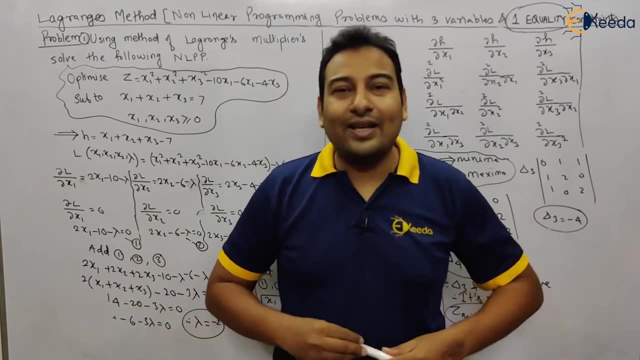 the. instead of minimum we would have written maxima hope. this is clear. the problem is exactly similar to the last problem or last time. you can say two variable with one equality constraint. it's just a bigger problem with few additions and you can easily manage the problem. 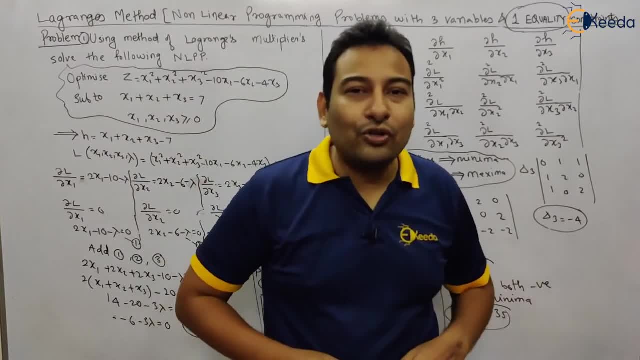 hope this is clear. if you have any doubt, don't worry. in the next video also, we'll be discussing example similar to this. thank you,